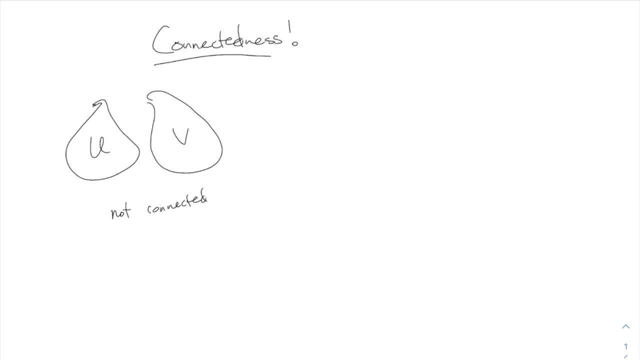 There's, you know, the U and the V. Those are the two halves in this particular picture, And there are properties that That the U and V have to have in order to be a separation. I don't think we need to review all the details today. 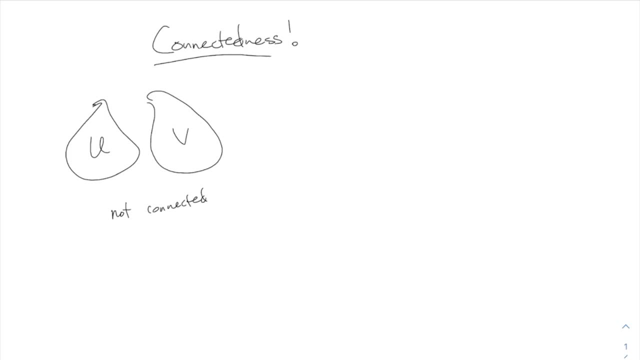 Last time we were talking about properties of connectedness and we talked about the fact that last time. So there's a theorem that said: if C1 and C2 are connected And something, something, something, Then C1 union, C2 is connected. 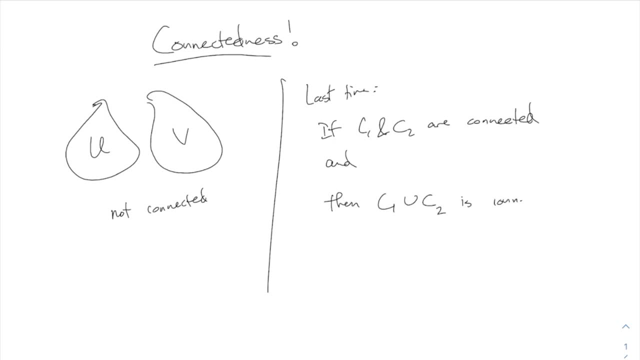 So the union of two connected sets is connected. All right, Anyone happen to remember the something, something Like this is not always true, that if you have two connecteds then the union of them is connected Because, like for instance right over here, 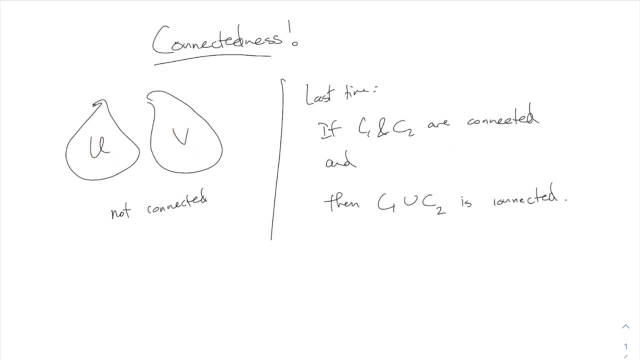 If I have two separate connected things and you consider the union, it's not going to be connected, Not always, at least. Here's two separate things, but considered together it's disconnected. Two things. it's connected. What needs to be true in order for it to be connected. 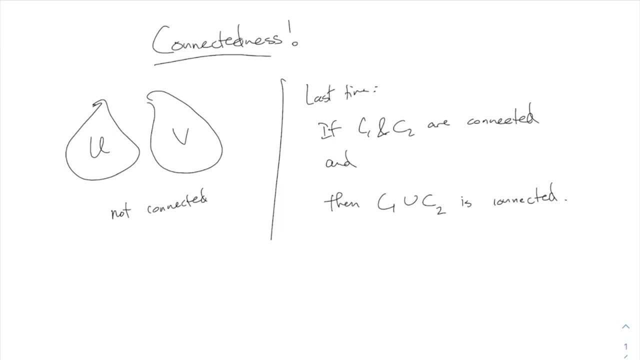 Yeah, Their intersections can be non-empty. Yes, They have some intersection, So the intersection is not empty. she said: So C1 intersects, C2 is not empty. This is the true fact that we ended up demonstrating last time, So that was a theorem from last time. 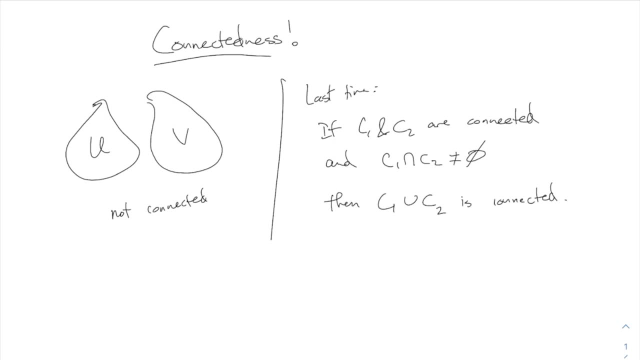 If I have two connected sets and they touch each other somewhere, their intersection is not empty. So that picture over there is an example where the union is not not connected. but if those two sets had one point together and they were still connected. 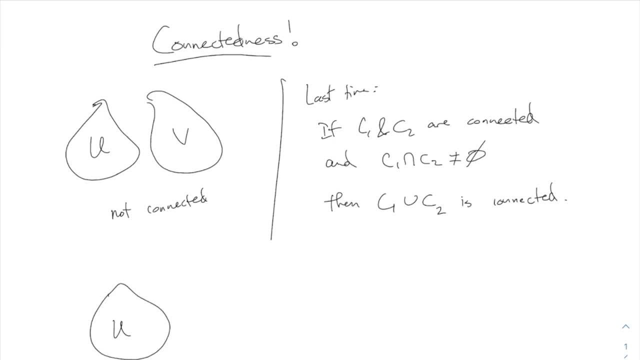 that would mean, you know, somehow maybe the U looks like this and the V looks like this. They have to touch each other somewhere. There's actually like a point in the middle. Well then, the union would be connected. 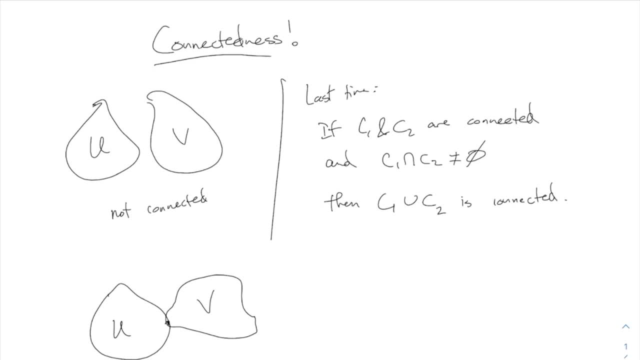 Yeah, So that's an example of when this kind of a thing really does happen. All right, Now we did. last time we talked about two connected sets, like in the picture, But actually this will work for any number of connected sets, not just two. 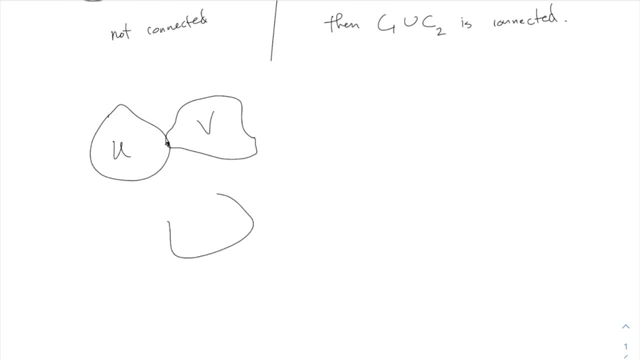 But if you add a third set in here, Now again, the third set can't be totally separate from the other two. It has to have something in the intersection. So you could do this with like a U and a V and a W, right? 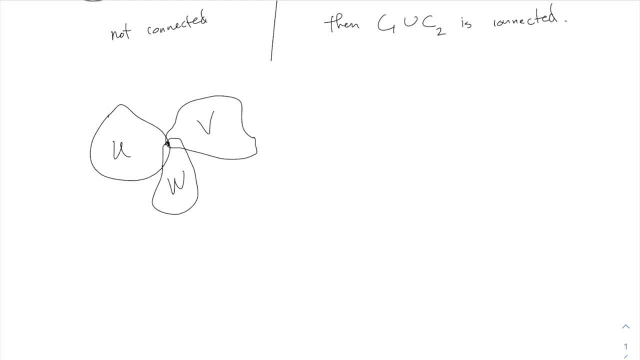 As long as all three of those sets have some non-empty intersection, then the union of the whole thing would be connected. Now you could probably actually say something like as long as any two of the sets have some intersection, but I'm going to go with all of them. 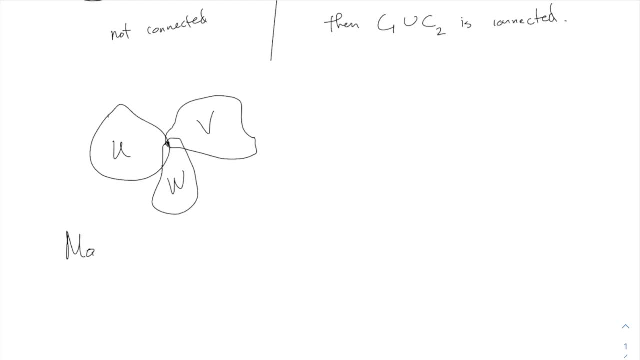 So there's a More generally, And this is better than what we wrote last time. More generally, we can have any number of sets, not just C1 and C2.. Any number of sets. In fact, it could be even infinitely many or uncountably many. 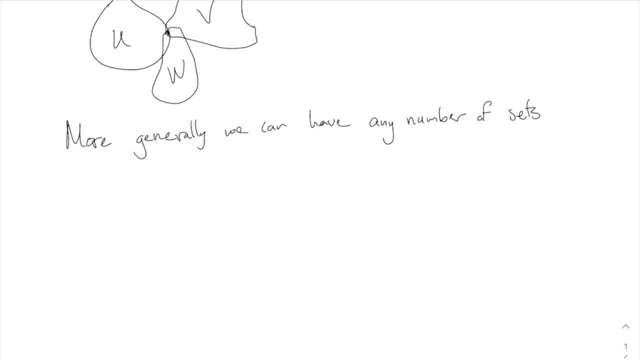 Actually, if you look closely at the details of the proof we used last time, it doesn't even matter if it's like an uncountable union. So, more generally, we can have any number of sets. So this is like the most general version of this theorem. 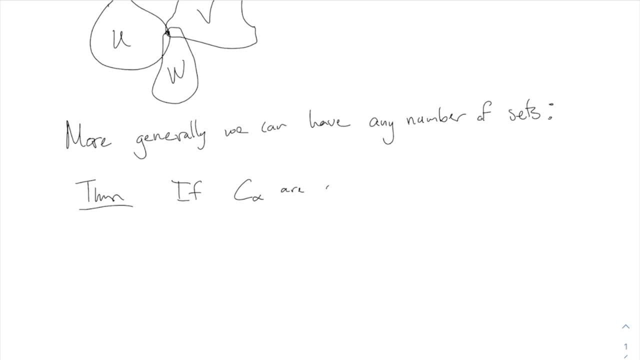 It says: if C alpha are connected, for all alpha in some index set A. This, remember, is how we have to talk about a collection of many, many sets, perhaps even uncountably many. You can't write like C1,, C2, dot, dot, dot. 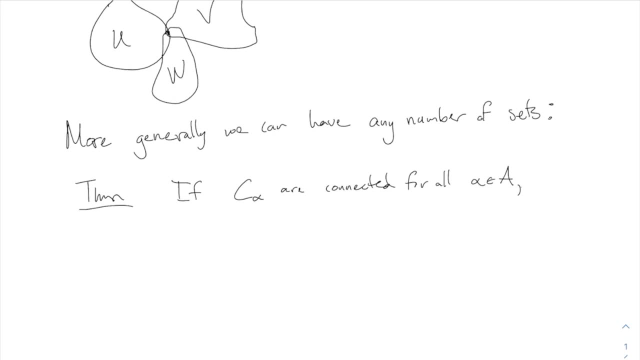 That still is. This is a countable number, But this is just any possible amount of sets. It could be an uncountable, Anyway, if they're all connected and if their intersection, which I would write like that, the total intersection of all of them- is not empty. 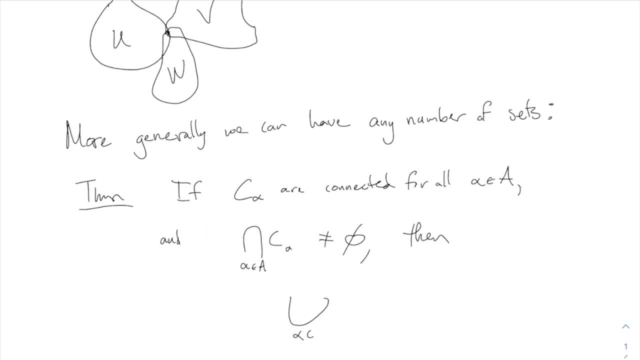 then the total union of all of them is connected. All right, This is kind of the full strength of that theorem that we did last time. We did it just for two sets, but it's really true for any number And it's the same proof that works. 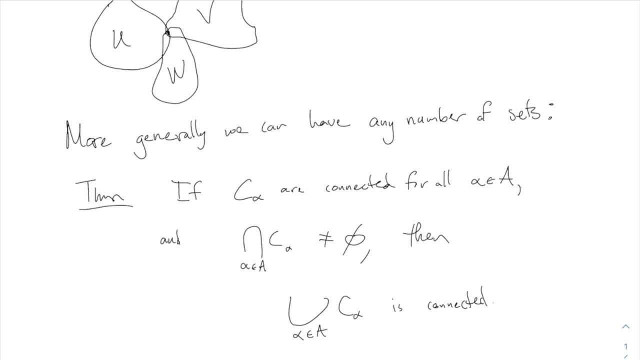 Although I don't want to get into the details of it again. All right, Connected- Any union of connected sets. as long as the intersection is not empty, the union will be still connected. Great, Let's talk the other thing from last time that I said I wanted to talk about. 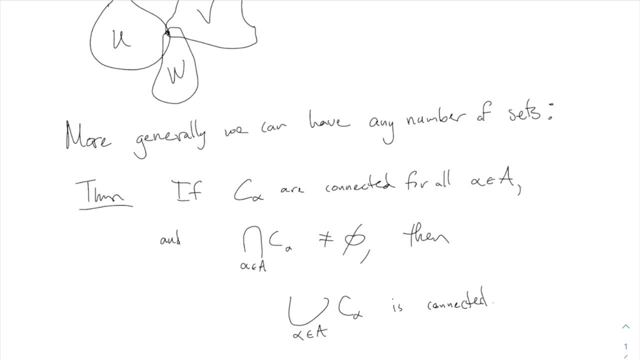 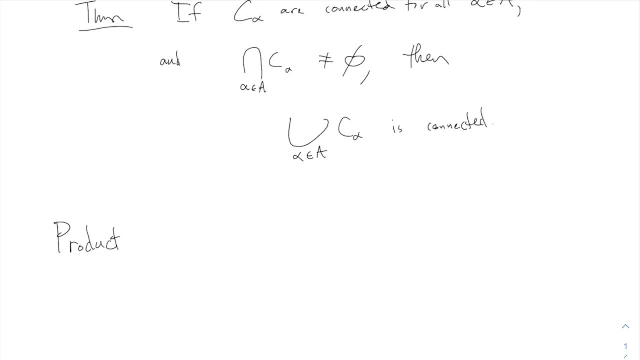 I wanted to talk about unions of connected sets and also products of connected sets. So this is the other thing that's kind of left over from last time. What about products of connected sets? I asked you to consider this. You know what if you have two connected sets and you take their product? 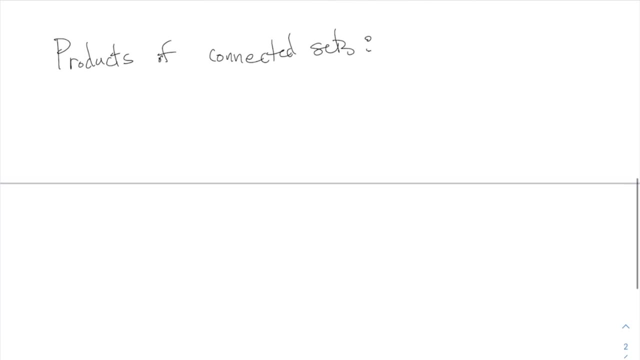 Is the product still connected? The way to think this through would be something like: if I'm in, say, a typical product would look like: maybe some set down here, some other, If I'm in another, set over here. if this is like, what do I call them? 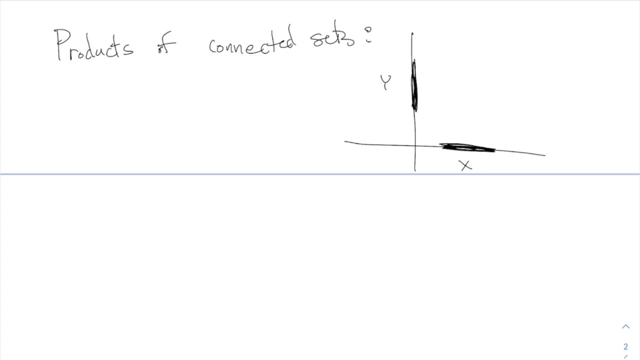 If I I'll just call them X and Y, If X and Y themselves are connected, and then the product in the picture like this: the product looks like sort of a box here, which is all this points, whose first coordinate is in X and the second coordinate is in Y. 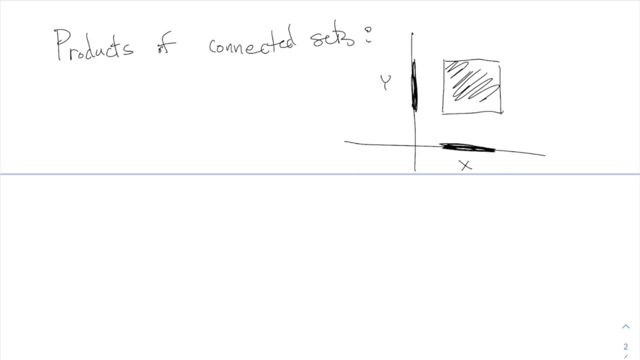 And I don't know about you, but it certainly seems to me that the product will also be connected. If the two pieces in the, in the two axes, are connected. it seems like the product will be connected versus if one of those pieces was disconnected, say if the X had two, two chunks to it. 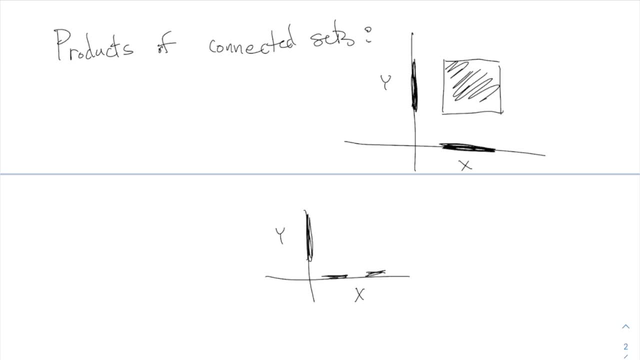 if this was the X and that was the Y, then the product actually looks like this right, And that is now disconnected. So it seems to me that the product of connected sets is also connected And that actually ends up being true. We have to. 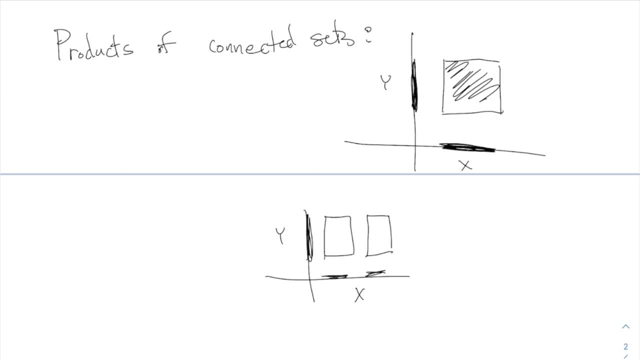 Demonstrate this, although this actually you can translate into something about unions. So anyway, the product of connected sets is connected. I'll I'm going to write that as a theorem. It says: if X and Y are connected, then X cross Y, the product is connected. 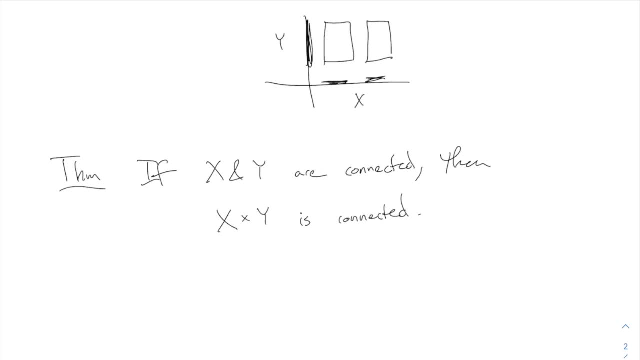 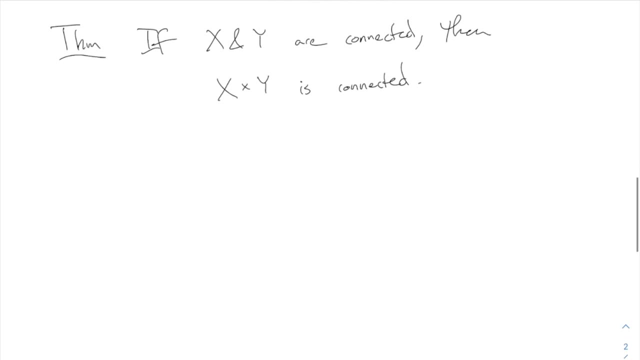 Here's a tricky trick. This is actually, in my opinion, a really cute proof. You imagine this picture Now, of course, I can tell just by looking at the picture. obviously it is connected, But this is a very specific picture. 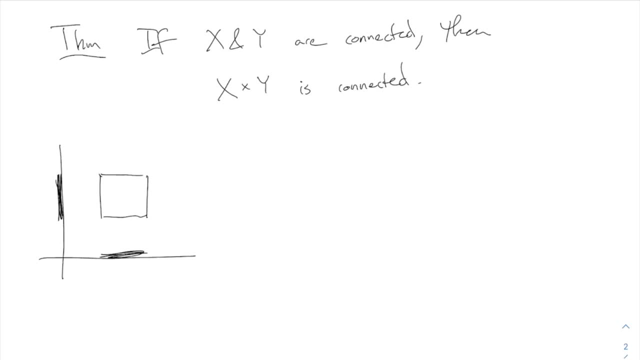 This is a picture when, basically, X and Y are both intervals. Everything works out nicely, But in general we don't. we don't want to assume that X and Y are all intervals. Here's the trick: The product. here the big trick is to write the product as a union. 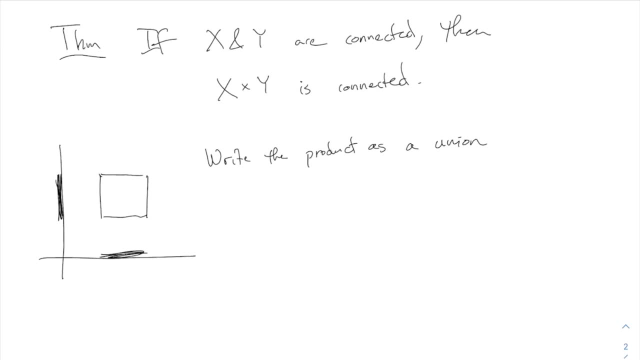 And then use the theorem that we had from last time about unions: Write the product as a union. I want it to be a union of connected sets. And what am I going to use for the union? Check it out. I could take a union, this product, which is this, this box here? 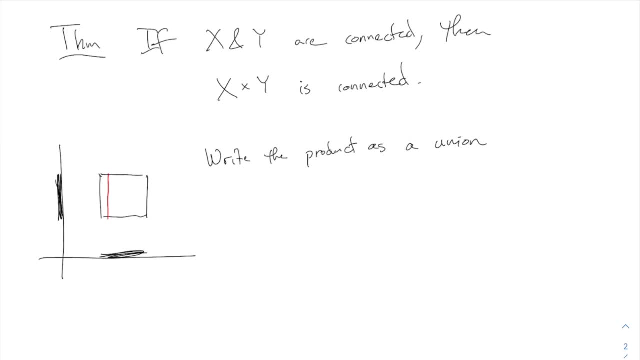 It really is a union of all of these vertical strips, So, like one of these vertical things, if I call this here, actually I'm going to do it. I'm going to do it. this, can I? sorry, I meant to do horizontals. 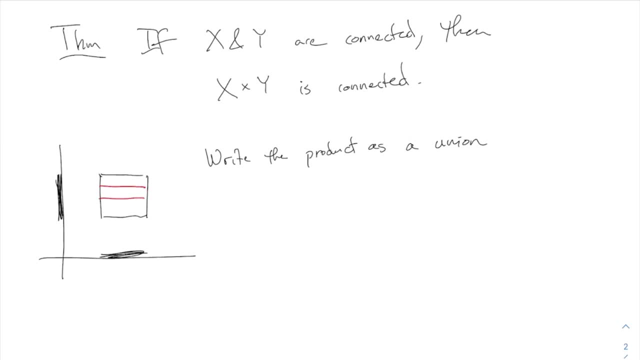 It doesn't really matter, but this is just the way that I did it on my paper. All of those horizontal bars, If you take the union of them, you get the whole product all right, And there might be, like in this picture, there's actually uncountably many horizontal bars. 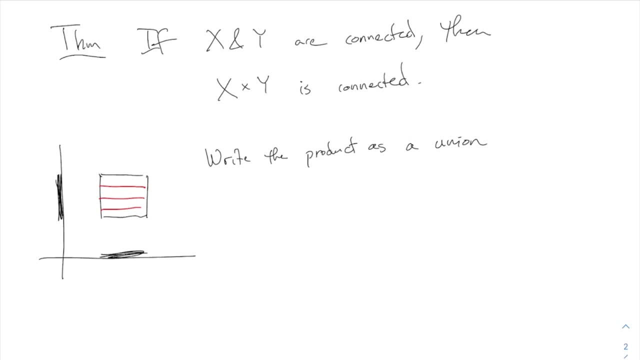 But it doesn't matter, because, because the theorem we just said, it doesn't matter how many of them there are. You can take the union and it will still be connected. Now, what do each of those bars look like? Each of these little sets here, each you know bar- you know what I'm talking about- actually looks like, you know. 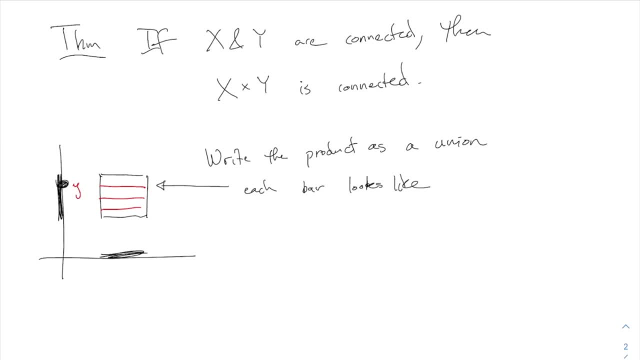 that one. Maybe it's y-coordinate, I'll just call y. It looks like- let's think about that- x cross just the point y. That is to say, you take all the points in the x-axis but you make all of their, all of their y-axis values, just that particular y value. 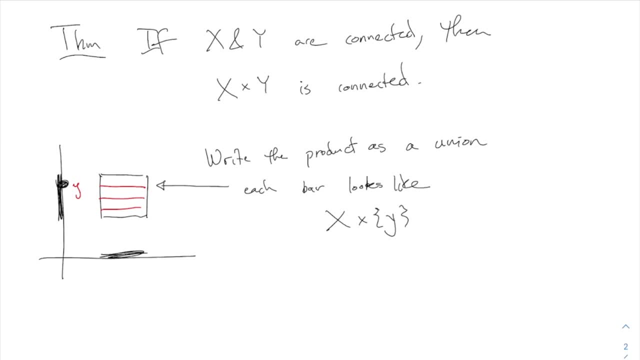 So each of those horizontal bars looks like the entire set x crossed with one particular y value, And that is connected. That's because this set is basically the same as x. It's topologically just a copy of x, but it's been moved up to some y position, all right. 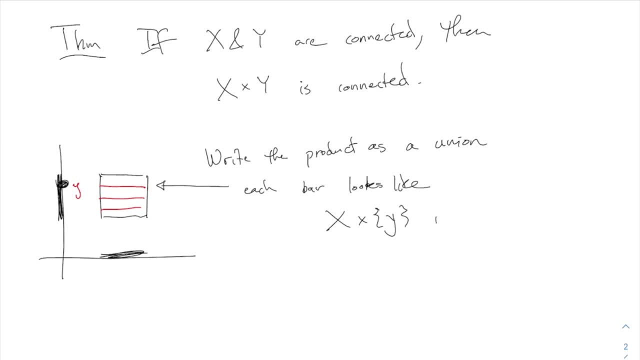 It, it. there's nothing else different about this. So this is connected, since it looks the same as x. All it is is it is just x, but it has a particular y-coordinate attached to it. But it is connected. 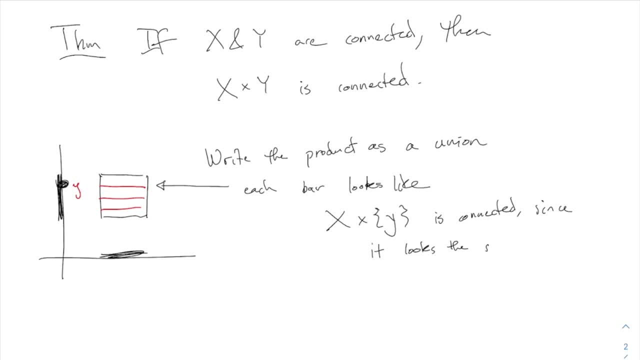 It's not changing the set at all. This is connected since it looks the same as x. all right, So each of those bars is itself connected, And then I can just take the union of all the bars and that will be connected. 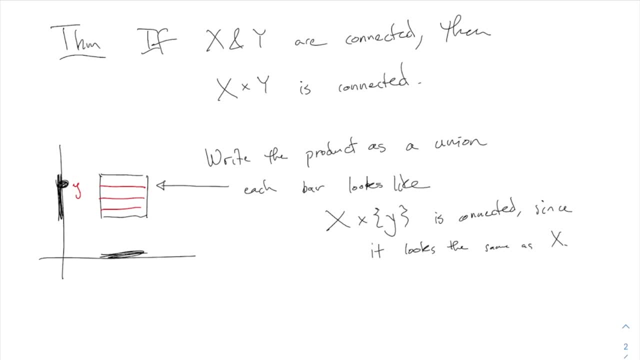 Actually that is not correct. what I just said I want to use the fact about union of connected is connected. Can anybody say what's wrong with that if I just take the union of all of these bars and I say it's connected? 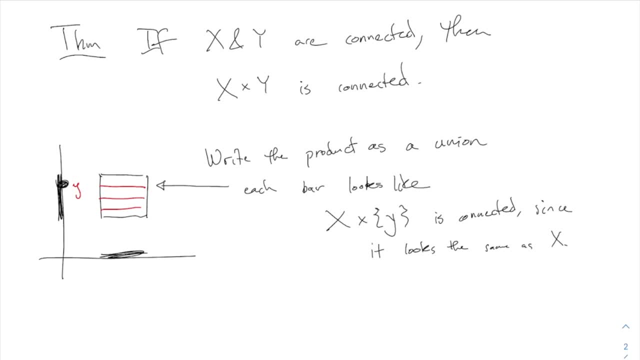 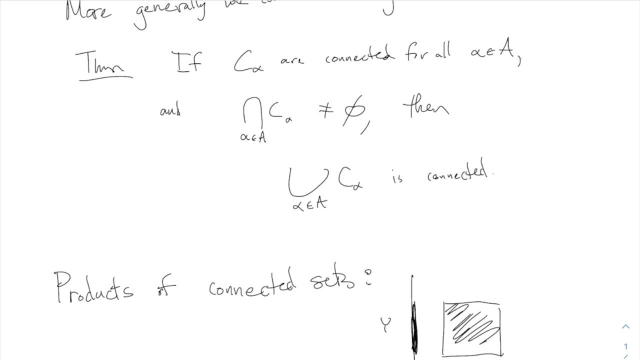 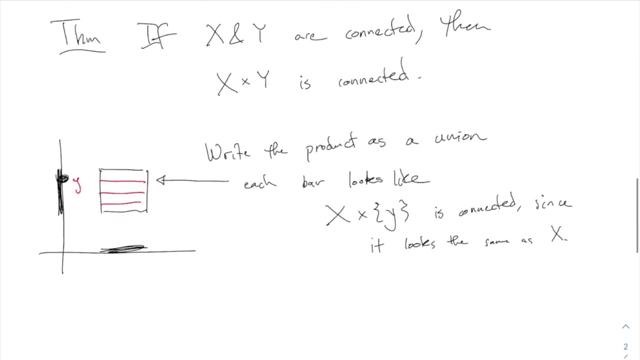 Because the union of connected is connected. You have to remember- I'm trying to use this, this theorem here- right, If everything is connected, then the union is connected. Can you see a problem with that? Yeah, these guys don't actually have any intersection. 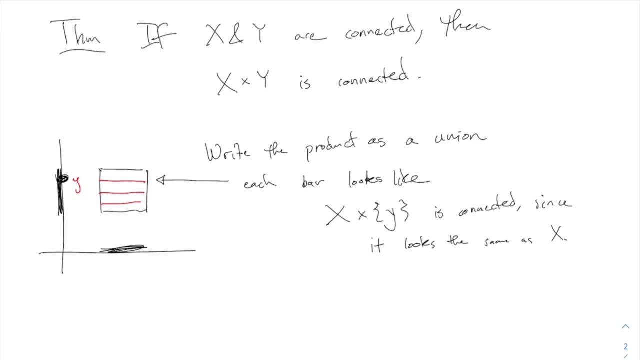 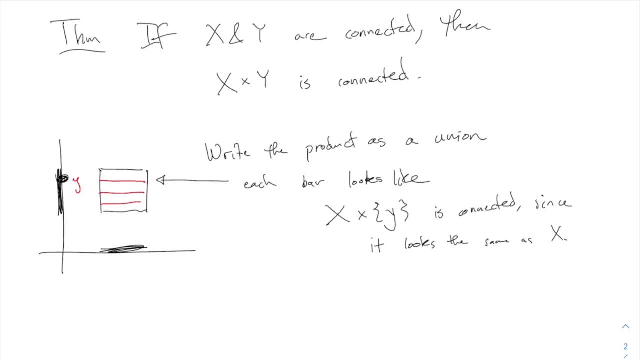 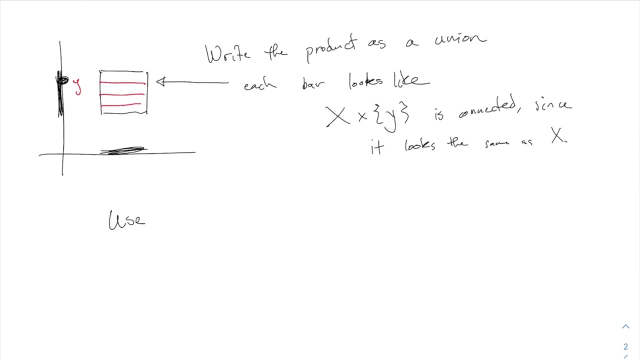 use that theorem because these horizontal bars don't have any intersections with one another. You can't use it as is. And here's the cute trick. The cute trick is, instead of these bars, we use crosses like this. So I'm going to choose one specific x value. 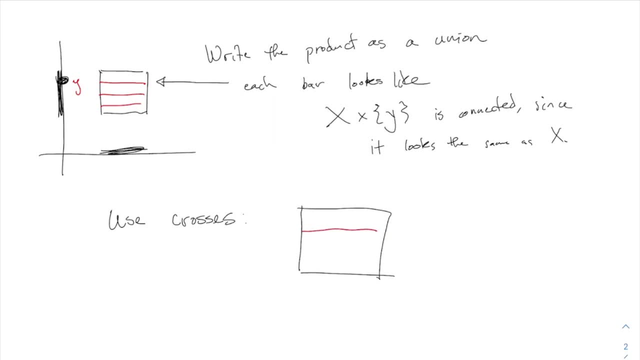 Actually, let's just use- I mean, on my picture maybe I'll just use the one furthest to the left. So I'm always going to use the vertical bar on the left end, but then I vary the horizontal bars that I'm attaching to it. 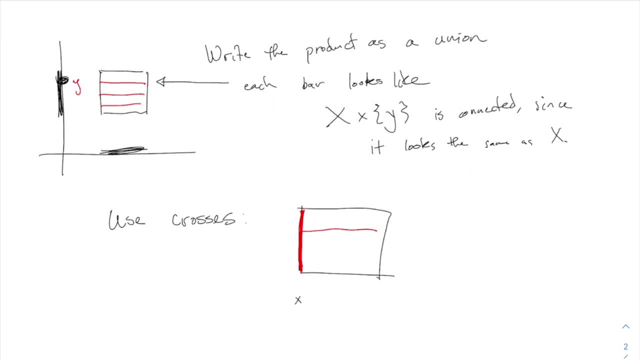 So if I call this, let's say, I have a specific x value down here, which I'll call x naught, and then these various y values up there. So this cross here, this is, it's a union of two things, right? 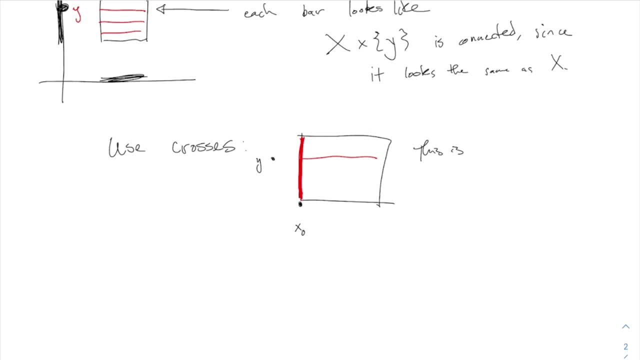 It's the vertical part and the horizontal part union together. The vertical part I could write as x0 cross y, That is to say, I use this x coordinate and then take the entire space in the second coordinate And then this is union, And then this is union with the horizontal bar. is like this right? 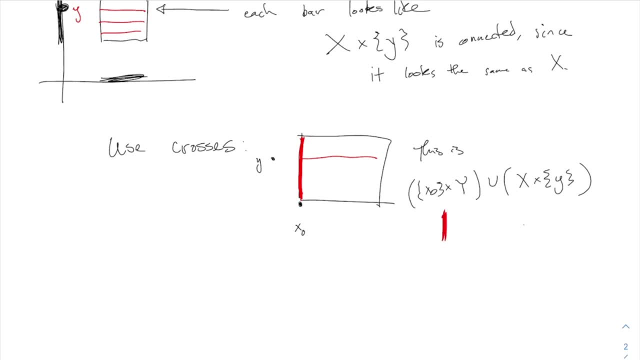 So this is the vertical part and this is the horizontal part. All right, Now that sort of sideways T shape. is that connected? Well, I wrote it as a union of two things. Each of those two things are connected Because this thing is the same as x. 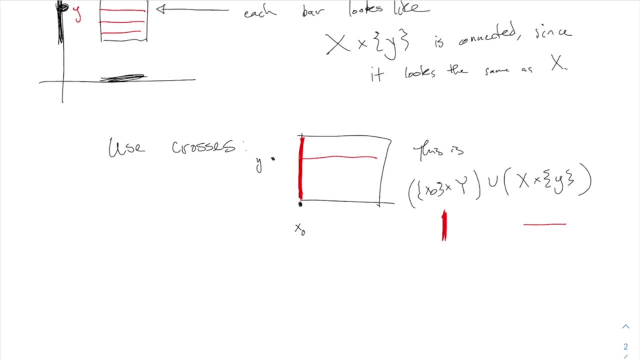 just with one another coordinate attached to it, And this is the same as y with another coordinate attached to it. So these are each connected. Can I use the theorem about the union of these two things is connected. It needs to be that they have non-empty intersection. 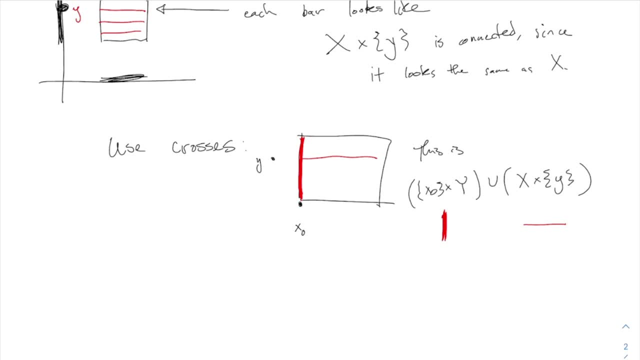 but they do have non-empty intersection because they meet at this point. Actually, you can say specifically what it is: It's x, naught, comma y, All right. So these two sets- I will say these two sets here- these are connected. 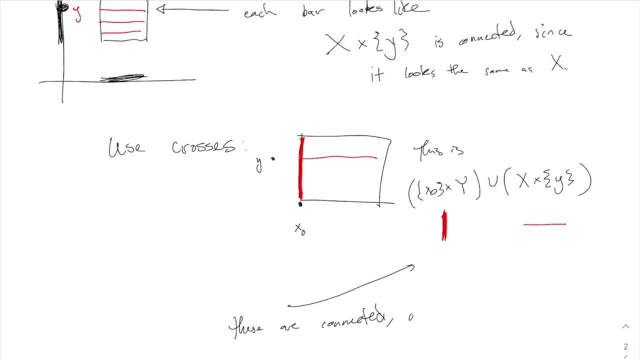 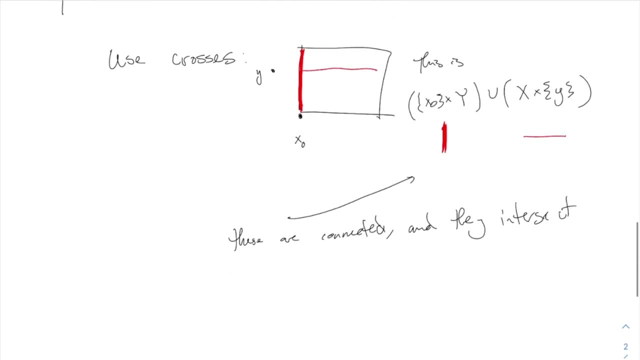 And they intersect. In fact, we can say very specifically where they intersect. They intersect at the point x, naught comma y. All right, And so that means this shape here is connected. All right, And now we can use the same basic idea from before. 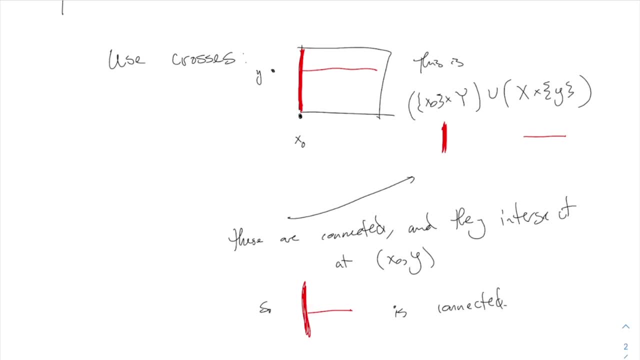 You take the union, You leave this vertical bar like it is, but union across all the different horizontal bars. And now the horizontal bars themselves do not have any intersection with one another, But if we always include this thing with them, then they do have an intersection with one another. 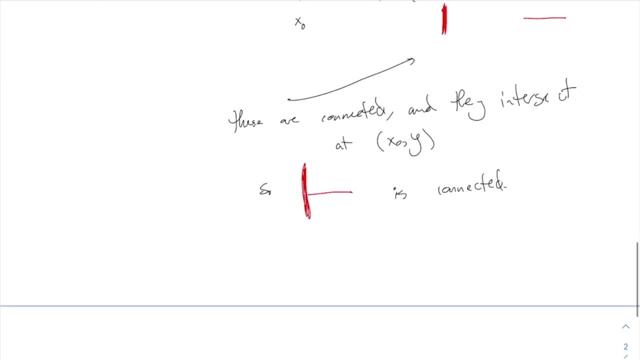 That's this thing All right. So we union take the union, So we have all the sets like they have. They all use the leftmost bar, but then they have various different heights. So it's like that, you know, like that, like that. 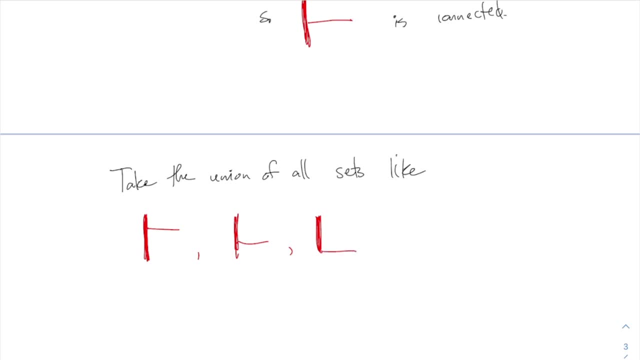 I suppose there's one at the bottom right, All the sets which use the bar on the left, together with a horizontal bar somewhere, And when we union those all up we get the entire product. So The union of all of these is X, cross, Y. 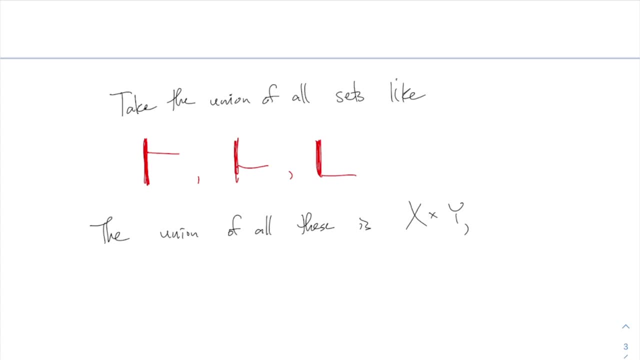 And they all have non-empty intersection. Their intersection, all of them together, includes the bar of points along the left side. All right, The union of all of these is X, cross Y and their intersection is non-empty. All right. In fact, specifically, it's that. 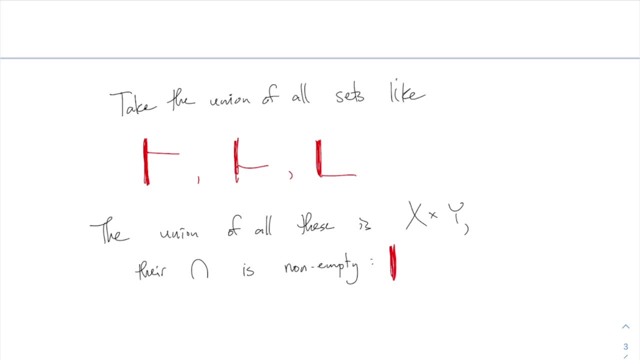 The vertical bar on the left. That's the intersection of all of them. So now we can use the theorem. We have a bunch of connected sets. They're individually connected. Their unions or their intersection is not empty and so their union is connected. 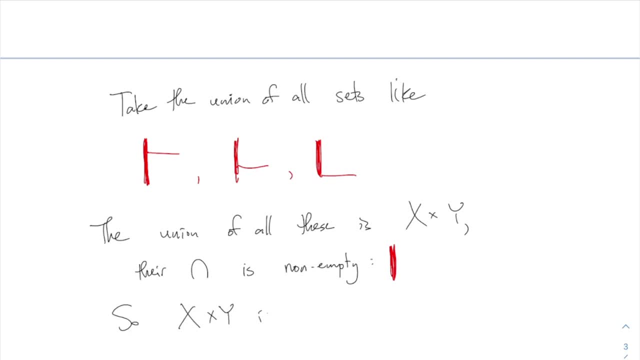 So X cross, Y is connected. That's it. This is the basic sort of Cute idea to write the product as a union of those kinds of things. It's not an obvious idea in my opinion, but it gets the job done. 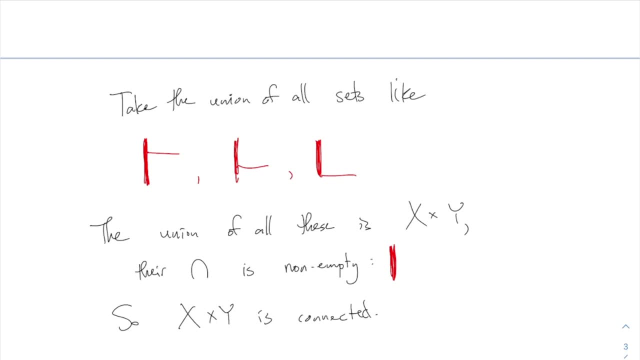 All right, Any thoughts about that? This is- I'm trying to sort of finish off what we were talking about last time- The product of connected sets is connected, It's true. All right, Let's discuss. Let's discuss one other thing from this section, and then we're going to move on to the next section. 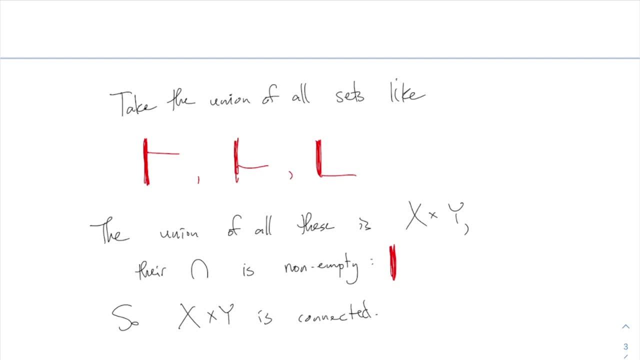 Actually, this whole first section has sort of a demoralizing title to this chapter. It's called something like a first approach to connectedness. There's actually much, much more to say about connectedness. I don't know if you feel like we've already said pretty much everything there is to say about connectedness. 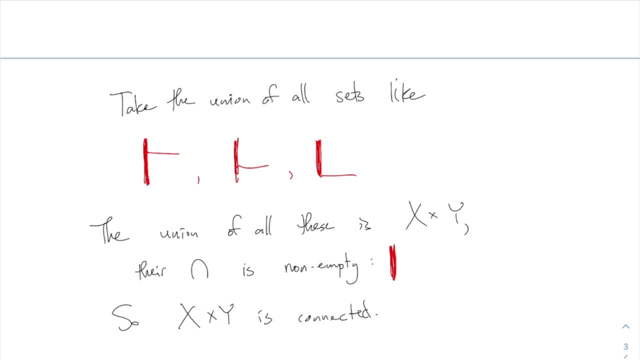 There's actually quite a lot more to say about connectedness, And maybe I'll give you a weird example just to sort of get your, Get your appetite going. This is something that we're going to talk in more detail about, probably next time. 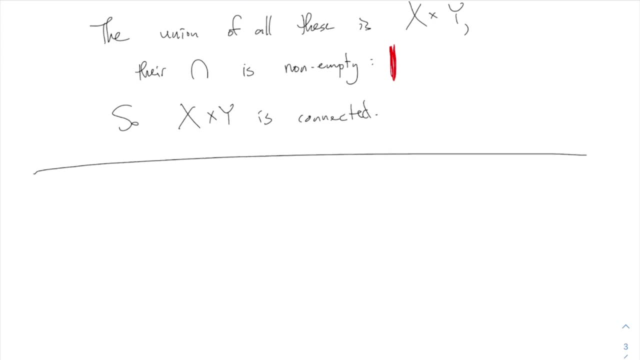 But just at this point to try to convince you that there are a lot of strange things that can happen when you're talking about connectedness. Check it out. Here's a not weird example Let's just talk about in R2.. Here's an example. that's not weird. 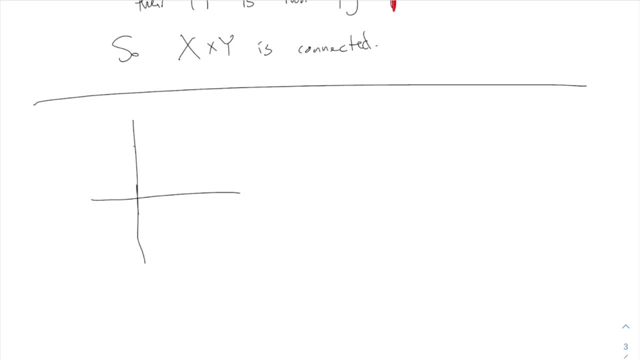 What if I have, let's say, this line segment like that? What would you say? Is it connected Or disconnected? This is not a trick question. The answer is connected. Yes, Just that interval. by itself, this is connected. 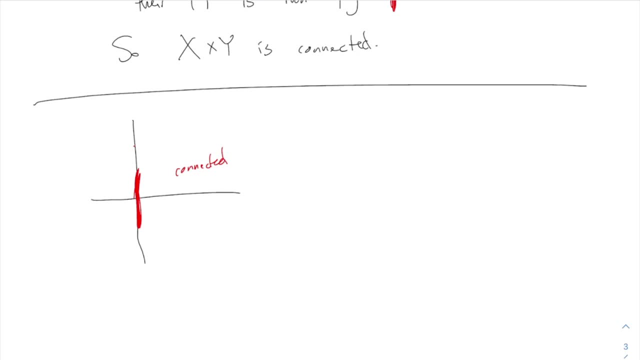 Okay, All right. What about two of them? You say disconnected. I hope you say disconnected All right. No funny business yet. There's going to be a little bit of funny business in a few moments, But let's, Let's try and make this slightly weirder, but still not really terribly weird. 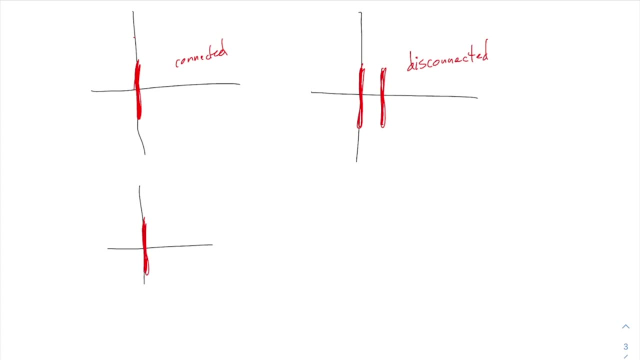 How about if these two bars, actually they do meet at a point at the bottom? Is this connected? now I say yes, this is connected. now, This is connected. Maybe Can I just say: I mean, it's obvious in this example, but why precisely is that one disconnected the two bars separately? 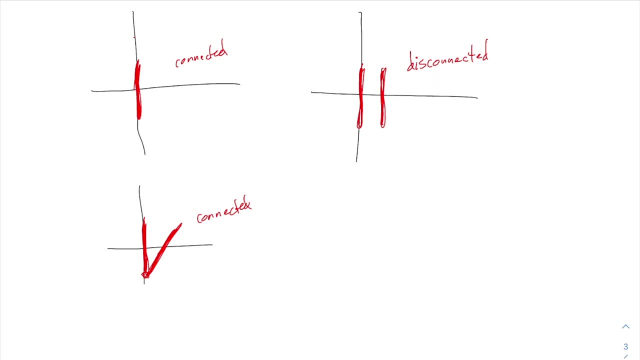 It's because you can make a separation Of that set by a U and a V. Now, since I'm talking about a subspace of R2, a separation in this context would look like something like a U is like an open set from R2 around this one. 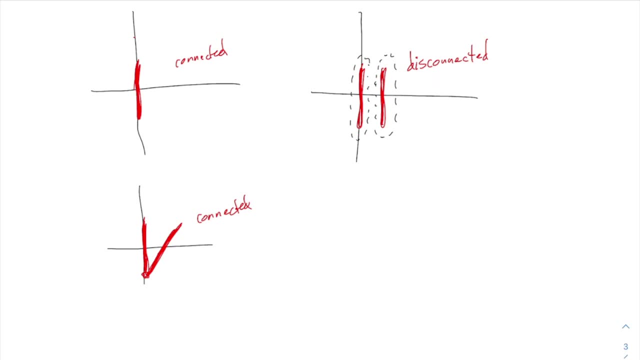 And the V would be an open set from R2 around that one. So this is like my U and V. That's what a separation looks like. This is disconnected because you can put open sets. The sets you use have to be open sets in a separation. 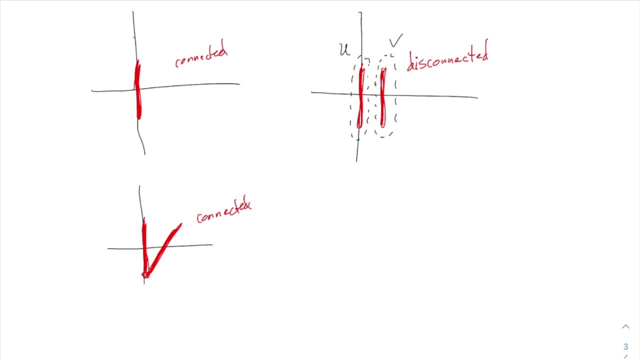 So they have to be sort of slightly- Can I say slightly- fat little worms around these two things. All right, And that's not possible. You can't do that over here without letting the two worms touch each other down here. So this is connected. 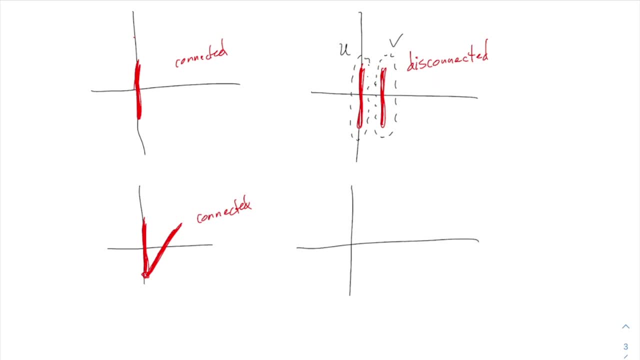 What about here's, maybe slightly less obvious. How about that same sort of V-like shape, but it does not include the point where they allegedly meet. Is that connected or disconnected? Disconnected, Disconnected, Yeah, Can you imagine where you would put the U's and the V's here? 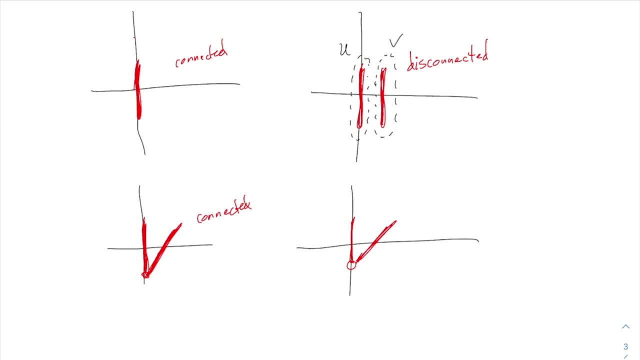 I mean I can, I would make The U's and the V's have these kind of dotted lines, outlines, So they are allowed actually to go right through that missing point. So in this case I could make the U some kind of wormy thing that actually goes right through. 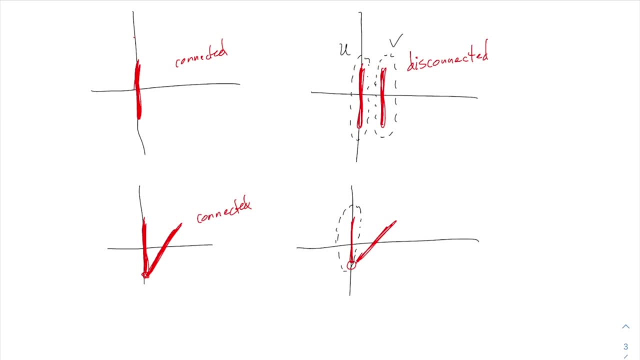 that point And I could make the V a similar kind of wormy thing. Now the U and the V are not allowed to intersect, But actually they don't have to. They can kind of kiss right at that point, which is being excluded. 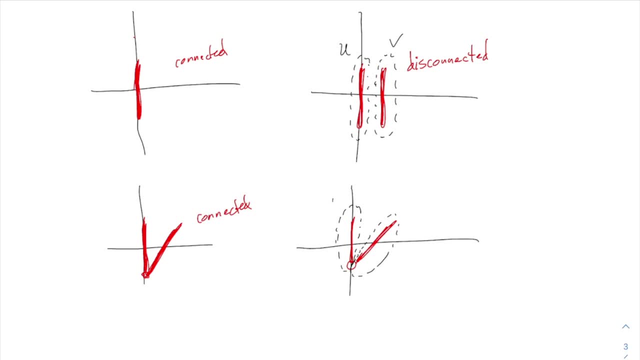 So there is really no intersection between the U and the V here, So this is disconnected, All right, Okay, One more None of these is the crazy example. Here's a crazy example. This is. you may have seen this. Actually, this comes up as a weird example in real analysis also. 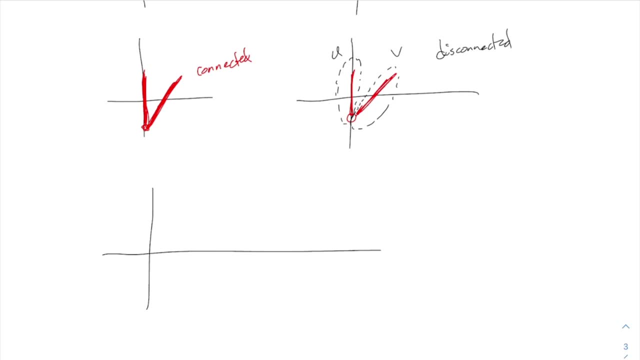 At least it is. At least, when I taught real analysis, I discussed this weird example. It involves this line segment plus another part which is a curve over here, And this curve- I want to oscillate like that- So actually this curve, so that, right, there is just a vertical segment. 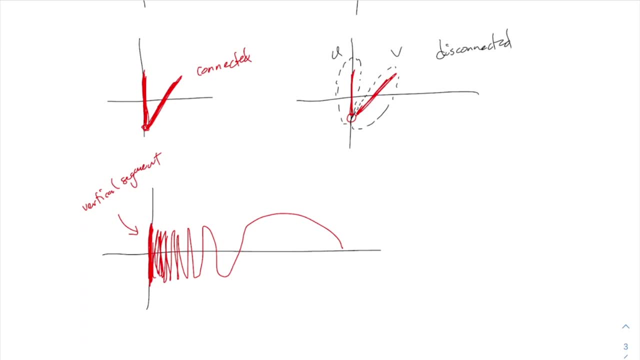 In fact, if you want to be very specific, you can say: this is actually as a set, it's 0, cross minus 1 to 1.. These are all the points where the x-coordinate is 0 and the y-coordinate is in this interval minus 1 to 1.. 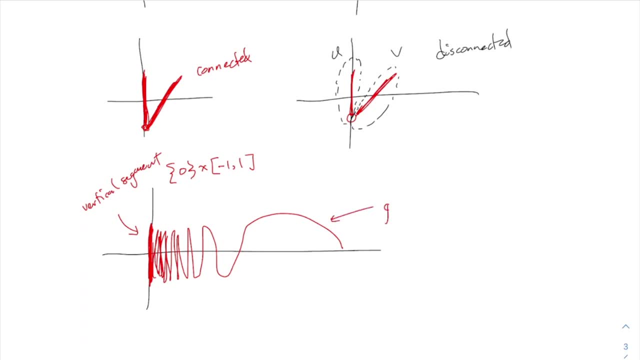 And then this part is the graph of sine of 1 over x. You can graph that on your calculator. You will see it looks like that. I guess I only want the right-hand side of it. In fact you could take the left-hand side of it also. 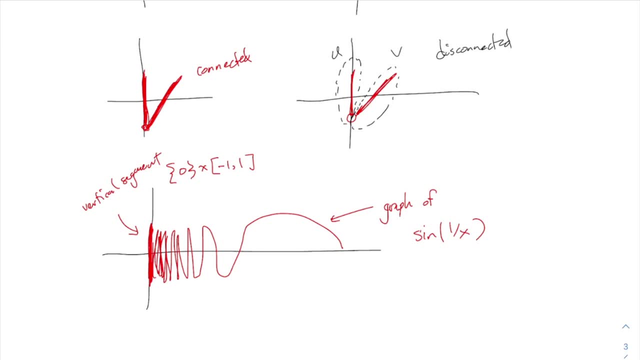 It doesn't matter. Sine of 1 over x. The way to think about this is: you know, the sine has oscillations forever. As you go out to infinity, the sine has oscillations forever. But because I'm putting 1 over x here, it's kind of like. 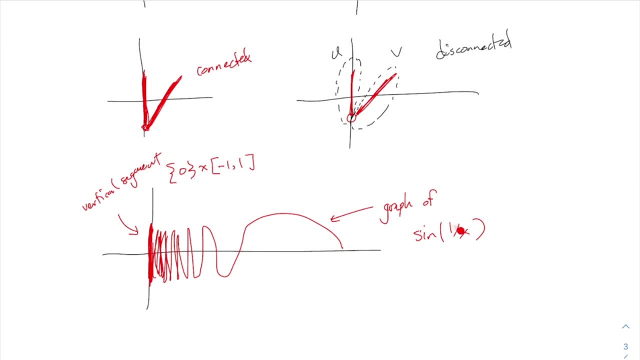 instead of going out to infinity, this thing, sort of all the business which happened when x becomes infinite. in this case, all that business happens when this ends up being close to 0. So as the x goes out to infinity, this goes out to 0,. 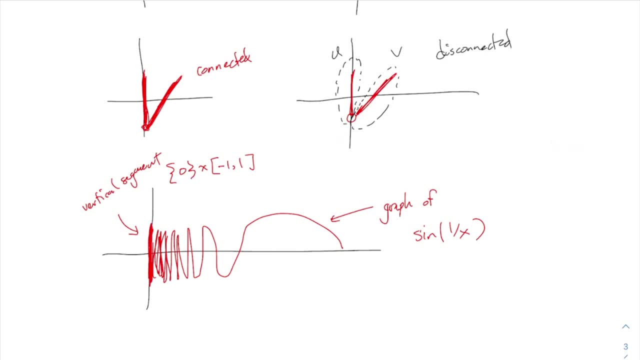 which means all the oscillations that usually happen on a sine as you go out to the right. all of those oscillations are packed into here as you approach 0. So it sort of oscillates infinitely often, All right. And I ask you, my friends, is this connected or not? 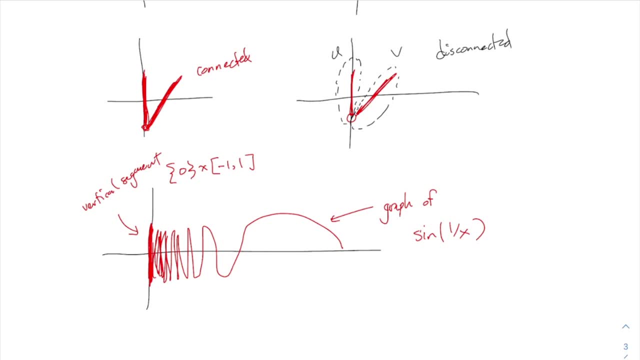 You have to ask yourself- I mean it does. I would say it kind of has two parts of it. You have to ask yourself: can you surround it with worms like u and v? And the answer is no, you can't. 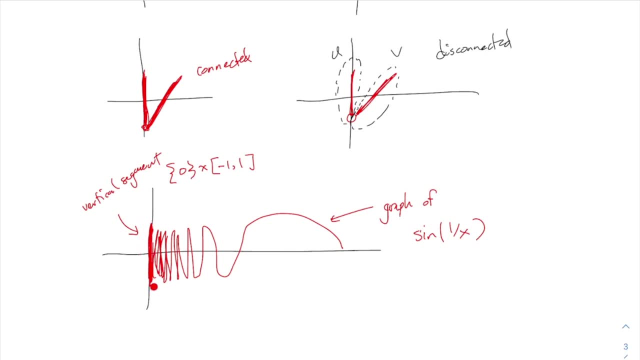 You can't put a worm around this vertical part without intersecting the rest of it. All right, So those. you could say they are two parts, the straight part and the curvy part, but actually they cannot be separated using open sets in this way. 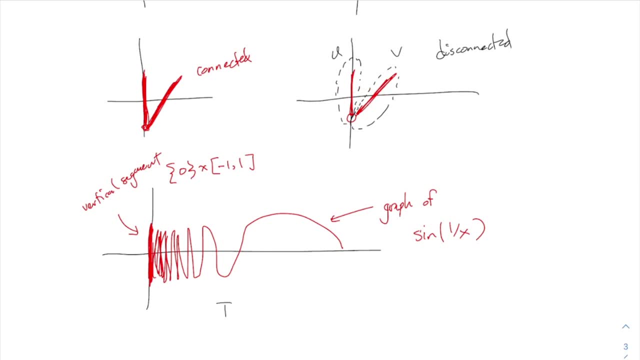 All right. So this here is connected, Even though it kind of does have two separate parts to it. I mean, it has the vertical segment and it has this curvy part. And if I asked you, does the curvy part ever touch the vertical part? 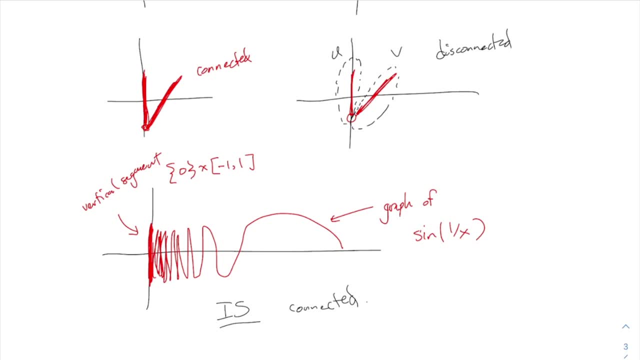 I would say no, not really. I mean, there isn't a point where this part touches that part over there. But according to our definitions, be it using separations or whatever, this one is connected. That's because you can't separate the two parts using 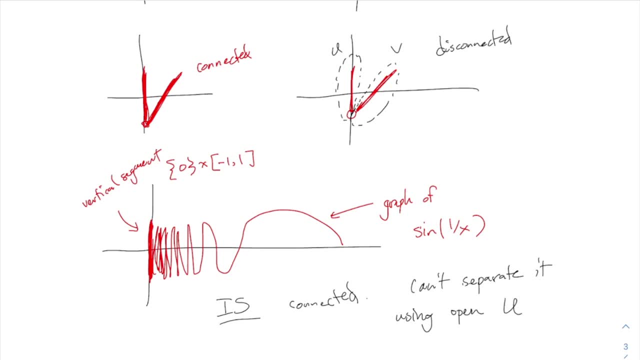 really it's because it has to do with the openness of the u and the v right. Since u and v have to be open sets in R2, they have to be sort of worms. They have to have some thickness to them And as soon as you try to wrap this vertical segment with some amount of thickness, 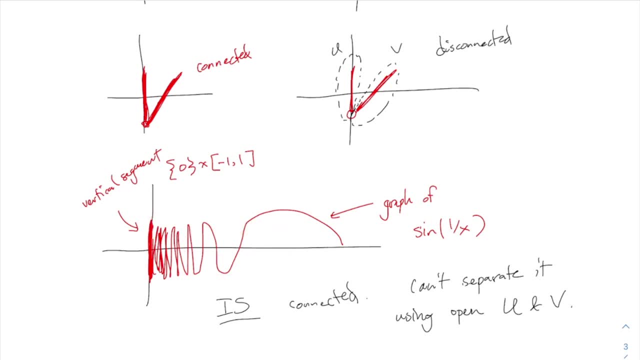 it will automatically intersect with this part. All right, So this one is connected, even though it kind of looks like it's in two parts. Another way of thinking about this is, if you were like a little guy walking along the road here, you can't ever get there from here, right? 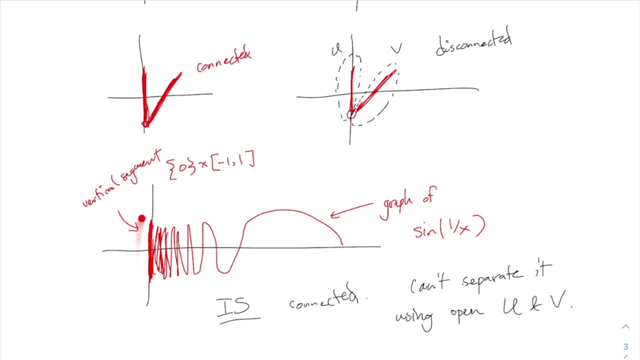 You can't walk from this part to this part. So from your point of view as like a little guy walking, you might feel like it's not connected because I can't get over there from where I am. But it is connected. It is connected topologically speaking. 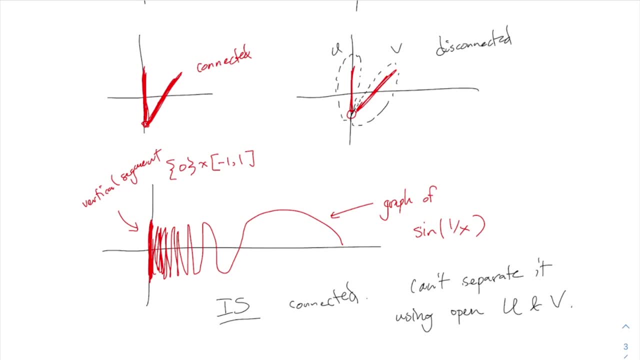 So actually there's another word for that, which is: if you're a little guy walking along, can you get there from here? That's something else. It's not called connected. So that's kind of where we're eventually going to go with this. 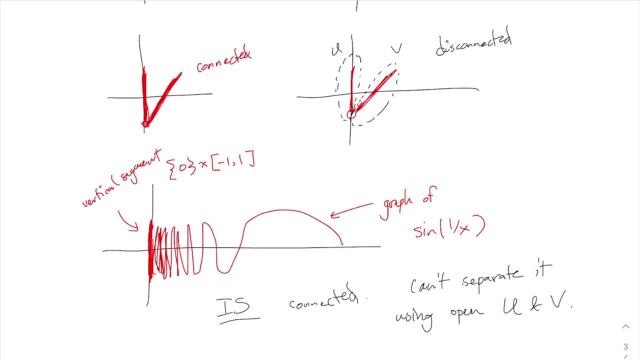 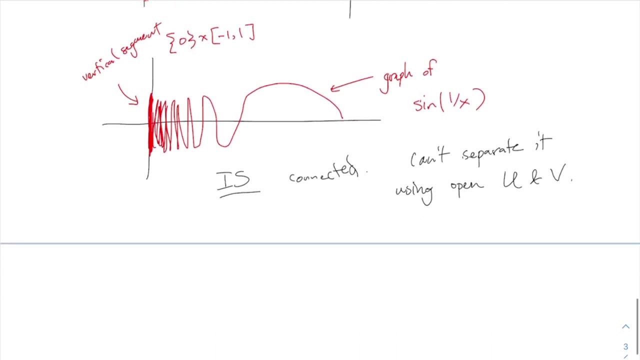 There are other types of connectedness, which in some cases are more natural ways to think about it, that are different from connectedness as we have been discussing it so far. All right, So before we get into these crazy examples- actually, the rest of what I want to say today is not really crazy at all- 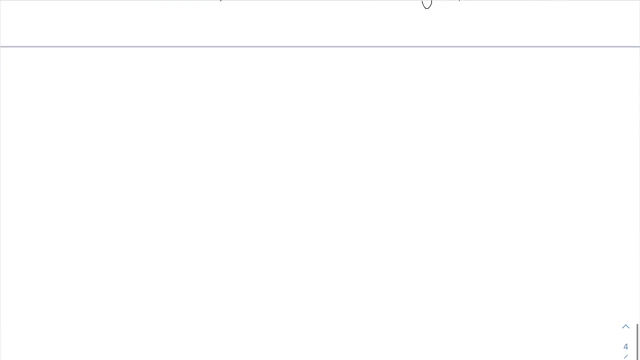 It's mostly ordinary kind of stuff. I would like to talk briefly about components, Components of a space. For some reason this word is sometimes pronounced components. I don't know why, because in ordinary English nobody would say that word Components, But some people call them the connected components of a space. 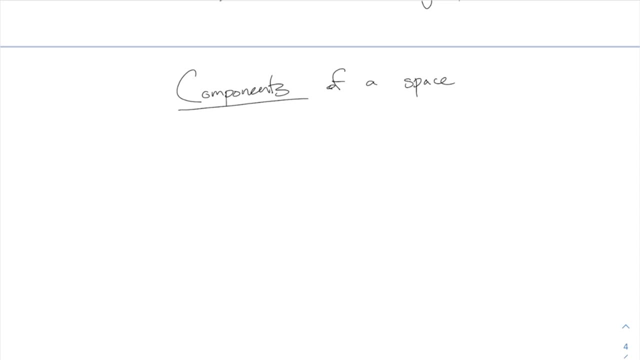 The components is what I'm going to say, The components of a space. This is just like, intuitively speaking, a very obvious idea. This is just like the pieces, If it's not connected, the pieces of a disconnected thing. Right, That's what I mean when I say components. 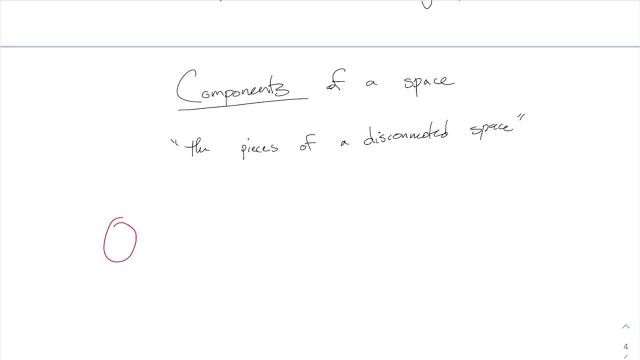 For example, if I have my space, is you know if X looks like? I don't know why I switched to red in two, maybe in three pieces. right, Here's X. How many components are there of X? The answer is three. 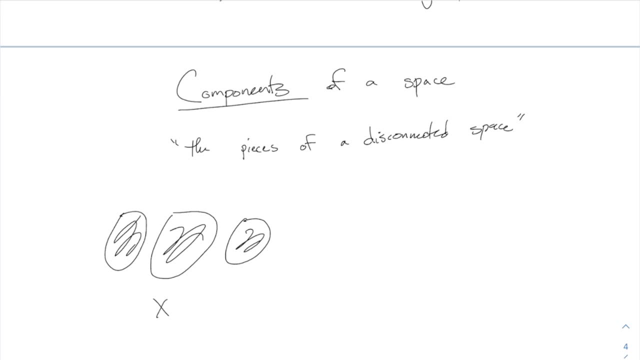 And what are they? They're those three things. Those are the components, All right, The pieces of a disconnected space. This has this right here- has three components, And they are those three sets. Those are the components, All right. 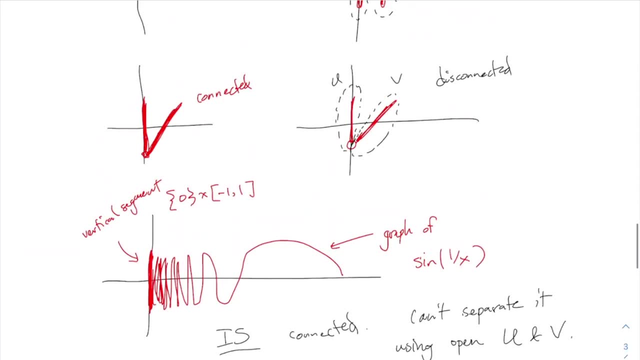 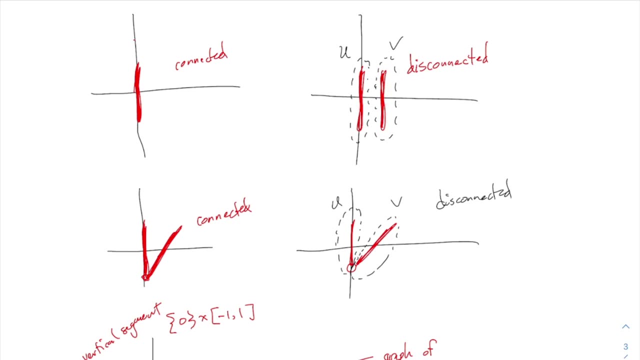 In these examples that we've been doing up here, right, You know, this set right here has two components. There are the two bars. Those are the two components. This one has one component, even though it feels like maybe it has two. 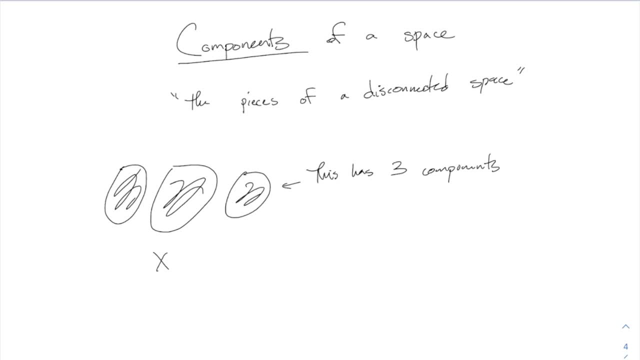 It technically has only one component. All right, This set has three components. I hope that this is an easy thing to understand. It is actually not so simple to define what exactly it means to be a component. All right, That thing has three different components. 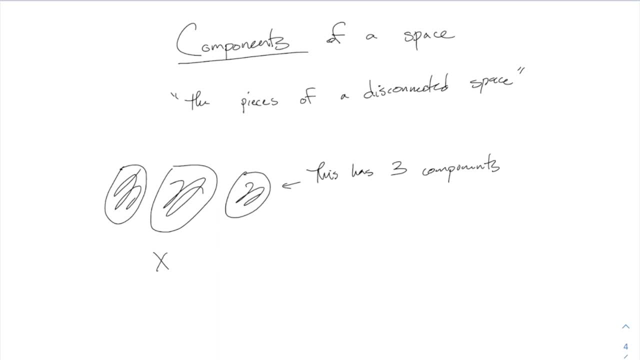 What is the definition of a component? It's a subset, Like in this example, each of these three blobs, by itself, is one of the components. So I want to write a definition. like you know, A, a subset of X, is a component. 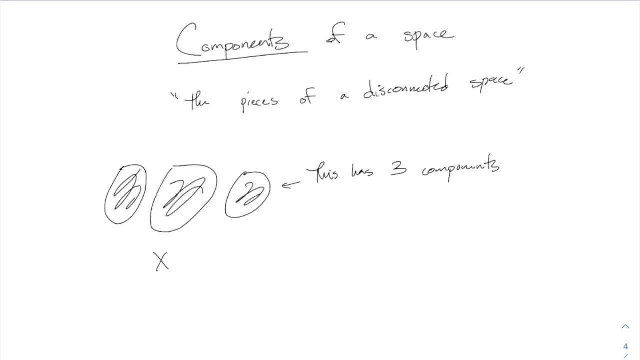 What does that mean? Anybody have a suggestion? Like when I say this thing over here is one of the components, What is that? What do I mean by that? Yeah, Okay, All right, This is great. I was kind of afraid somebody would say like, well, you know, it's like one piece, like one chunk, all alone. 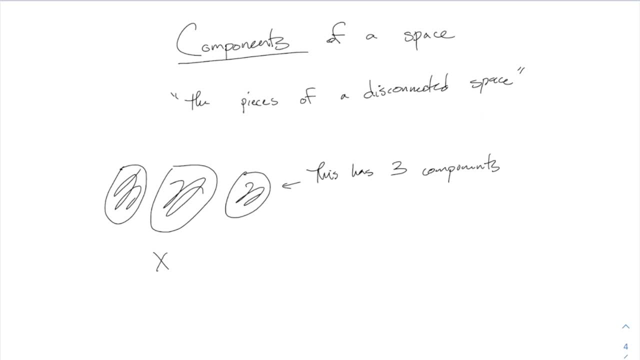 This is not the kind of answer we're looking for. I said something better, which is, first of all- this is important. He said the component by itself is connected. Right, So you don't like those two things together doesn't make a component, because those two things together is disconnected. 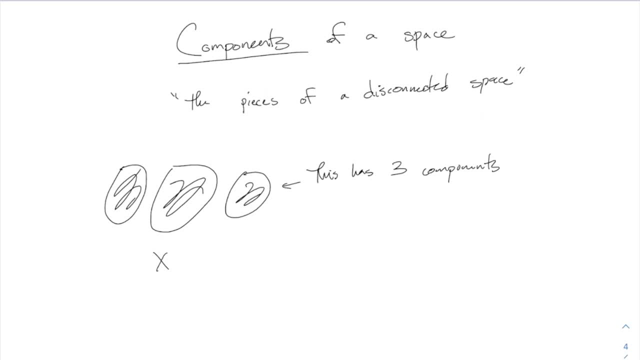 So a component all on its own is connected. That's not good enough, though You can't just say that, because, for example, then I could take: I mean, just like a single point inside of one of those, Like one single point by itself is connected. 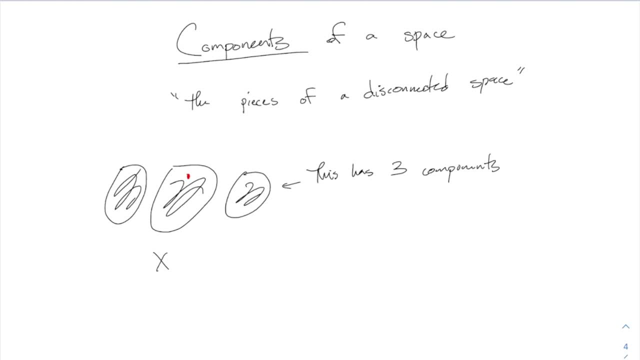 But it's not a component Because it's sort of not big enough. All right, What else is required? So I think he said it's connected by itself. and what else did you say Disconnected from the rest of it? Yeah, 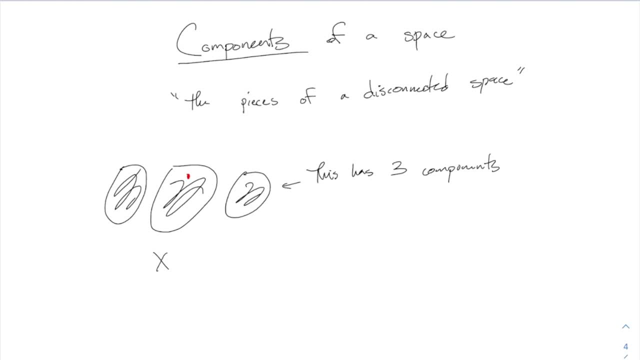 I'm not sure I like that phraseology. Can anyone have a better way of saying that- And this is actually not easy at all, in my opinion, to say in a better way than that Disconnected from the rest of it? You have to be a little more specific about that, maybe. 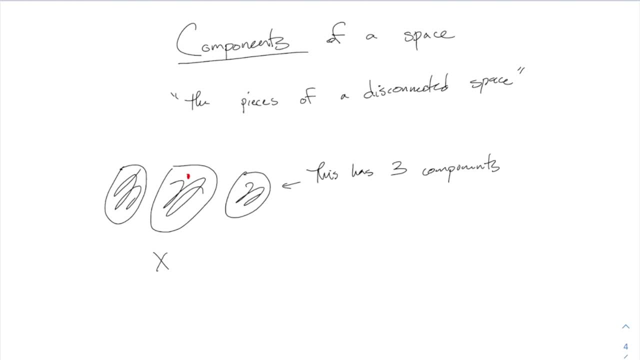 Actually, here's the way that this is done in the book. There's actually a few different ways that you can make this definition. They all end up being equivalent, But the way that our book does it is actually. they don't even try to define what a component is to begin with. 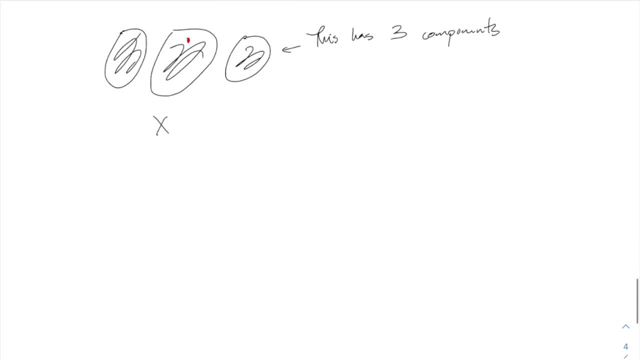 It turns out. this is a strange but true fact. It's hard to say, Can I just say: Hard to say exactly what a component is. The definition has to be a little complicated. Hard to say what a component is, But it's fairly easy to say what it means for two points to be in the same component, versus two points being in different components. 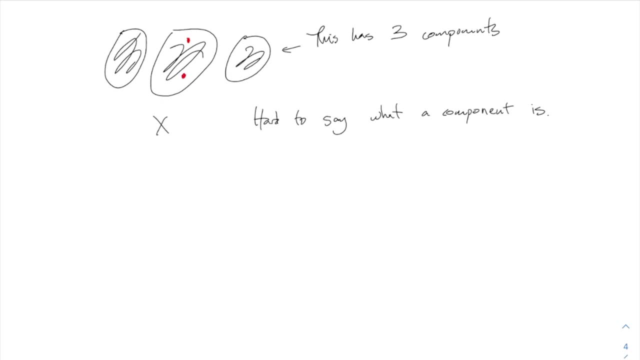 For example, those two points, the two red points, are in the same component. That actually is easy to define. So we can define: x and y are in the same component, Even though I'm not saying what the word component means. but I'm giving a definition for what it means for two points to be in the same component. 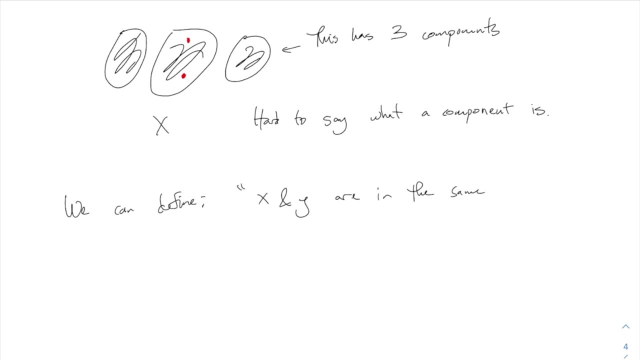 X and y are in the same component And we're going to write this as x, Like a little. it's a relation: Some of the points are in the same component as one another, Some of them are not. And the way that our book, our book, writes it with this tilde, with a little c. 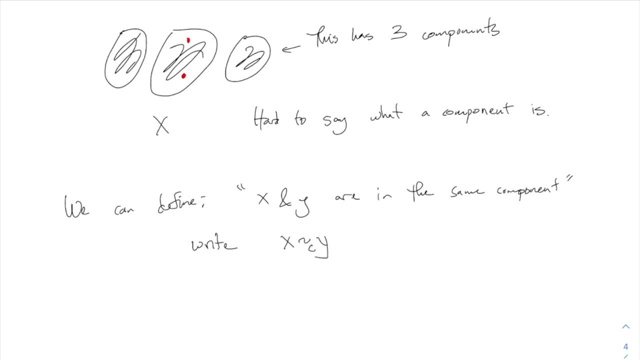 I imagine the c stands for component, or maybe connected, I don't know. X and y are in the same component. We write it that way. Anybody want to suggest how can we like give a real definition of the fact that the x and the y here are in the same component? 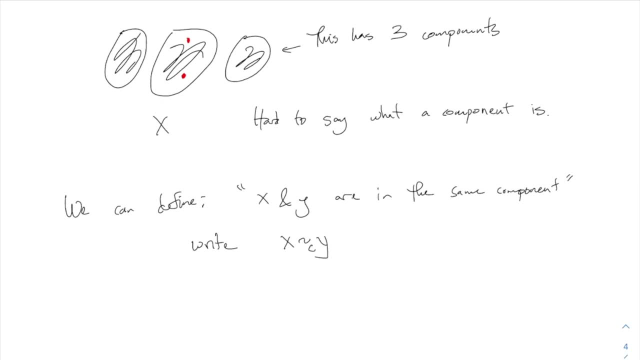 This also, I suppose, is not obvious, Although once you see it it's not so hard to say These two points are in the same component versus. you know, this one over here is in a different component from those two ones. Why is that? 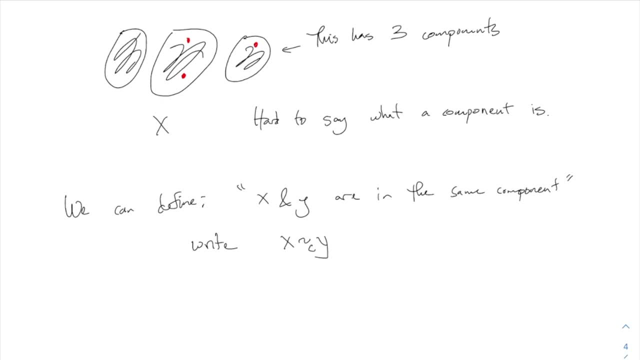 Maybe I'll give you a little hint. These two guys over here You can. Those two guys are inside a connected set. There is a connected set that contains both of them Versus this other one over here There isn't. You can't make a connected set, say, from that one which also includes that one over there. 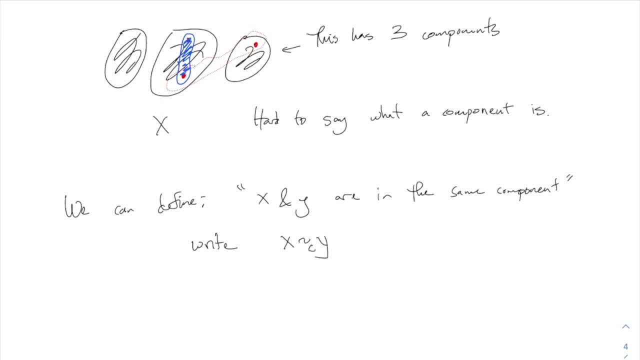 Because? well, because they're in different components, But that's the definition of this. So I'm going to write: x is equivalent to y when x is in the same component as y. when there exists a connected set, I will call it a, with x and y both in a. 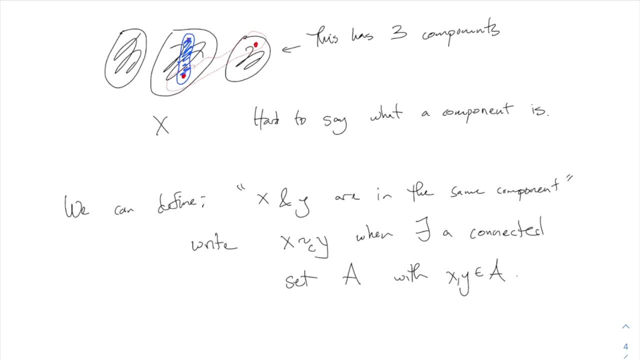 If that's true, then the x and the y must be in the same component. Even if you don't know what the word component means, You can talk about this relationship here. You might feel like I'm defining. I'm using a term that I'm trying to define. 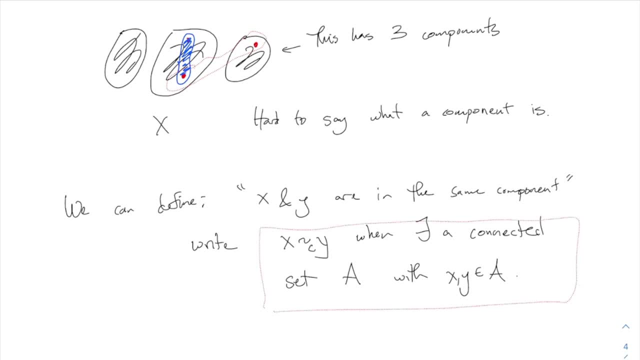 This is the real definition of what I'm talking about here. All right, X is equivalent to y when there is a connected set which contains both of them, And then the definition of a component is: it is the equivalence classes of this relation. So certain of the points are over here. 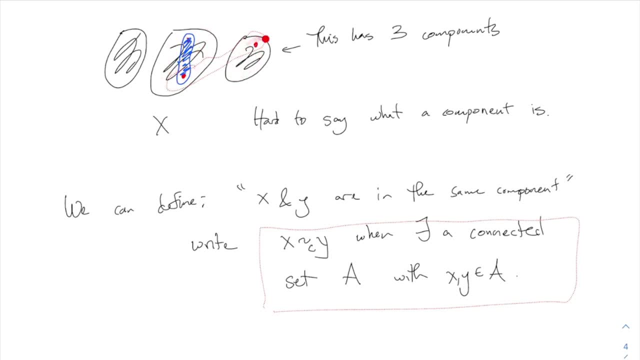 That's one class. Certain of the points are over here. That's another class. Certain of the points are over here. That's another class. And those classes are the components. That's the definition of the components. This is kind of complicated. 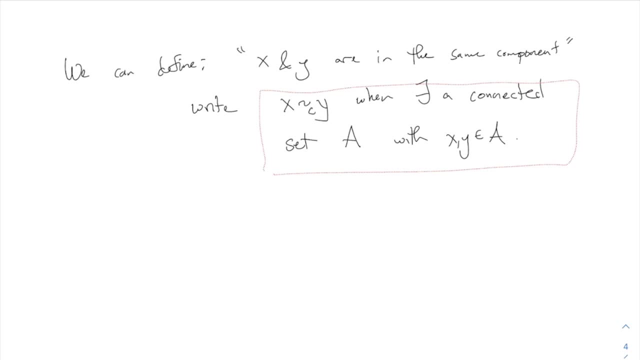 But there isn't really a much easier way that you can do this. So- and actually I don't even want to go through all the details of this, But it turns out this is an equivalence relation. This actually you have to prove. It's not so hard to prove. 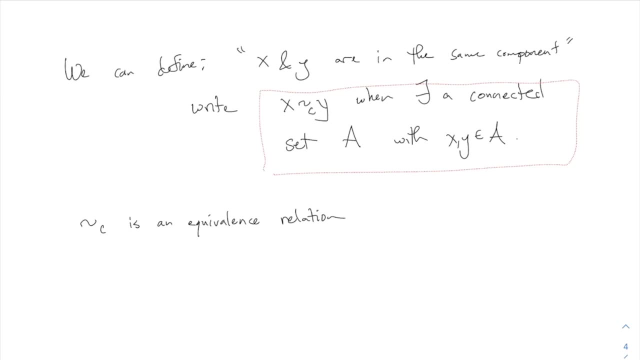 But I don't want to get into it. It's obviously reflexive X and x. You would have to show that x is related to x. That is to say, is there a connected set which includes x and also x? The answer is just: x as a point by itself is a connected set which includes x and also x. 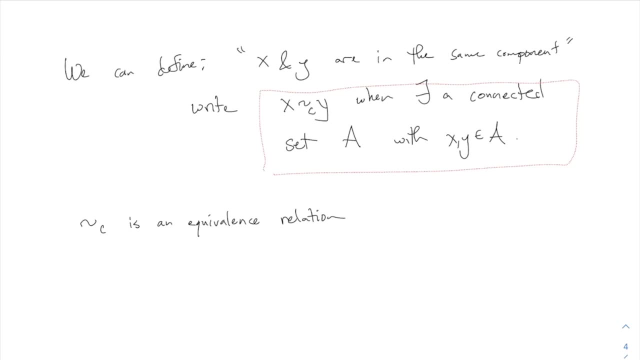 It's also symmetric And the transitivity is a bit of a pain, But I don't want to get into it. Anyway, this is an equivalence relation And then the definition. this is the true definition of components. So a component of x is an equivalence class. 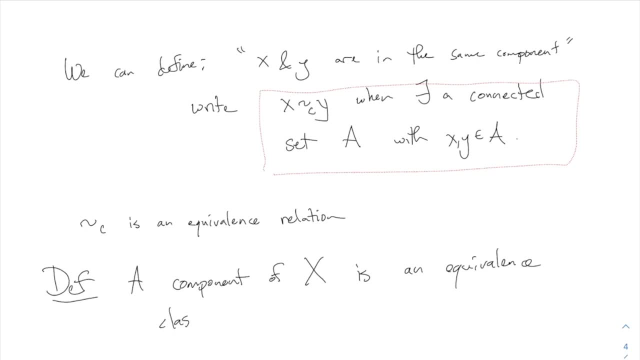 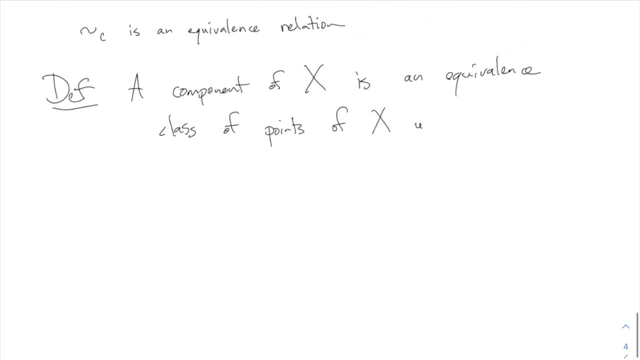 Of points of x Under the relation This guy. All right, This, in my opinion, is a very confusing definition, But there really isn't a much simpler way to do it. All right, It is an equivalence class of points of x under that relation. 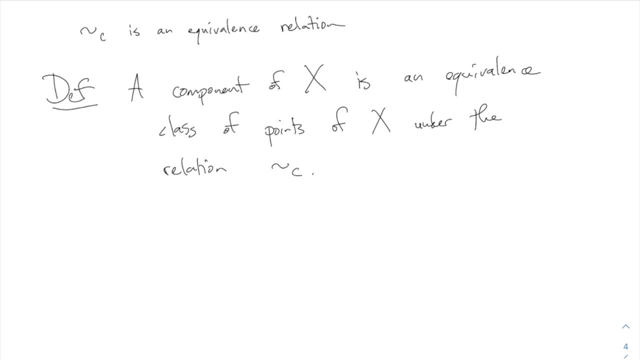 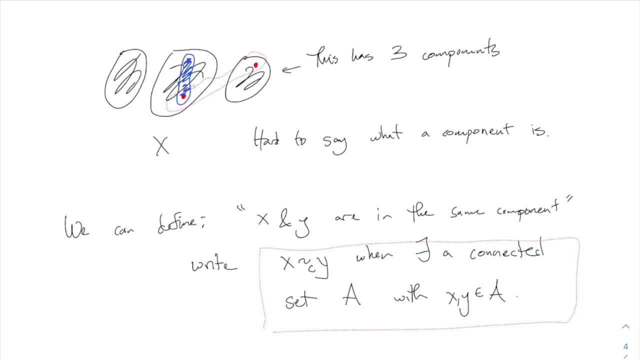 So you look at your set as a whole And you ask yourself: where could the points be, if they are equivalent to one another or not? And the answer is: there's some points in this part, There's some points in this part And there's some points in this part. 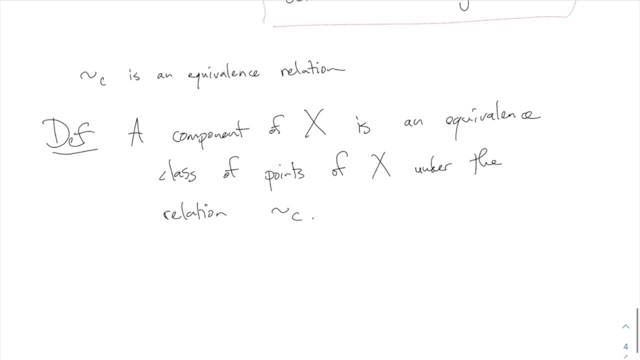 Those are the three different equivalence classes of points. All right, Those are what the components are. Maybe I'll tell you. I said there are several different ways of making this definition. Here's another one. This is an equivalent one, Which I don't. 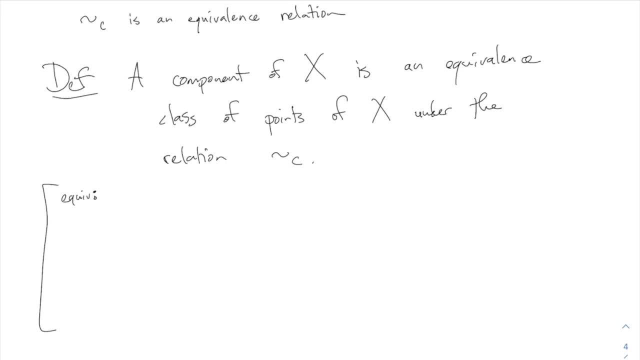 This one actually, from a certain point of view, in my opinion, is a little easier to understand, Although it's harder to use, And so we're not really going to use this version of the definition, But it says: if you can understand all the words here: 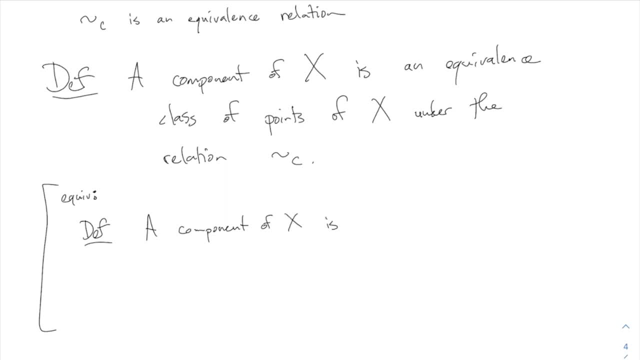 A component of x is a maximal connected subset. I think this may be closer to what Alvin had in mind before. A component is something which, first of all, by itself it is connected, And then this word maximal Meaning it will not be connected anymore if you try to make it any bigger. 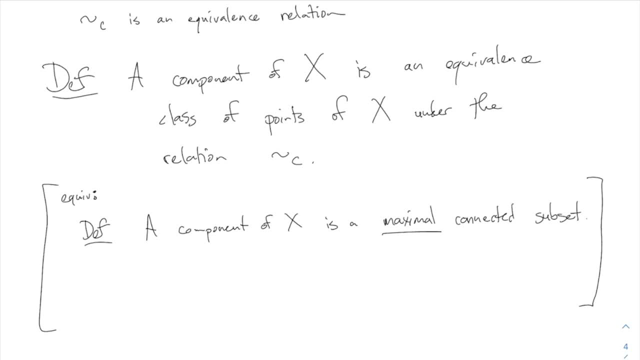 You can't get a bigger connected set than the components. So the picture is sort of If you have, If you imagine a picture like maybe this part, And How about just like Two half open intervals Going like this Right. 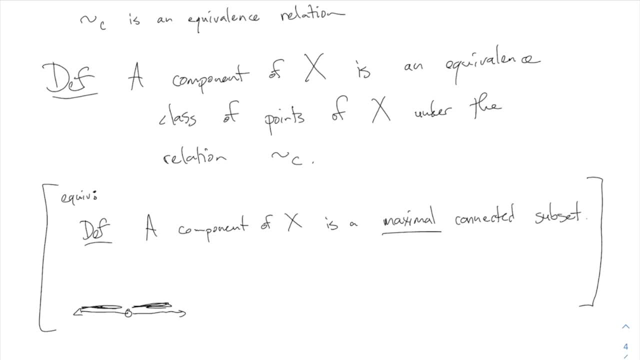 This is one component And that's another component. What it means that those two things are the components is, First of all, each of those two things are connected by themselves And also, if you try to make them any bigger, They would. They would fail to be connected anymore. 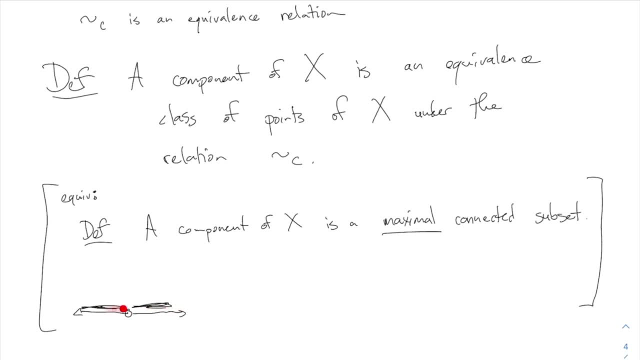 Like this set over here. If I tried to grow it out to the left at all, You can't include that point. So if you, If you, included any more of those other points, It would become disconnected. That's what this maximal means. 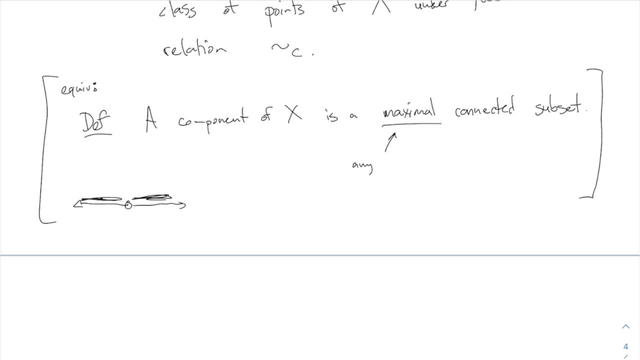 It means that Any larger set Would be disconnected. All right, I think that this is This is not so hard to understand the idea, Although it's It's a. It's kind of a pain to use this as a definition. 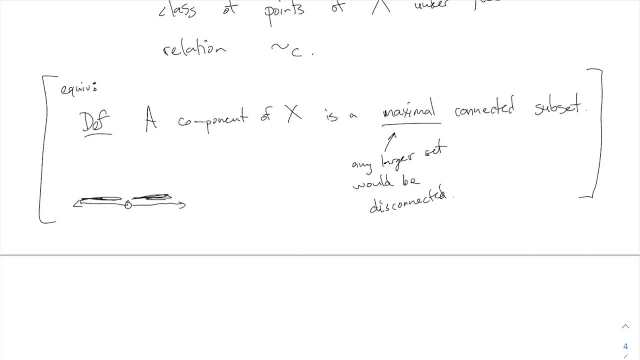 Because you always have to talk about this maximality thing Which is technically Difficult to use in practice. All right, Anyway, I would like to do some fairly simple examples of I show you a thing And then you tell me what the components are. 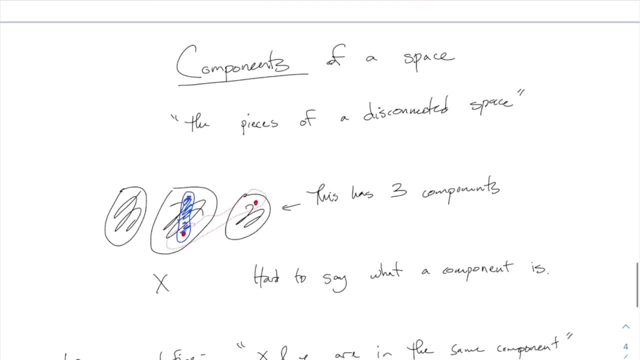 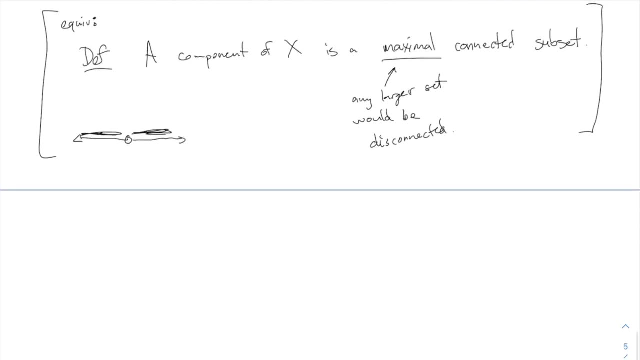 Now, if you can just look at, If you're just looking at shapes, Then it's pretty much always obvious what the components are, Although we can I have some slightly more interesting examples than just that one. Let me just say, To summarize here: 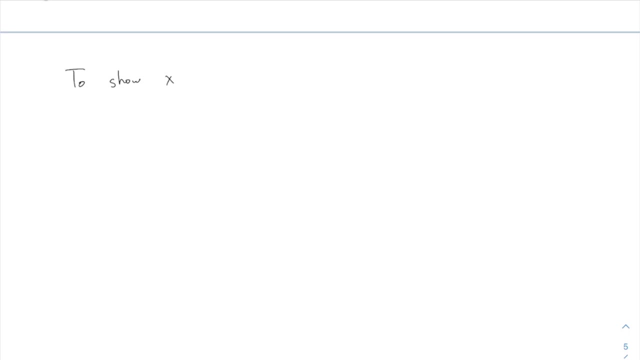 To show that Two points, Say X and Y, are in the same component. This is easy. Typically You just Give a connected set That they are both in All right. This is how you would show that Two different points are in the same component. 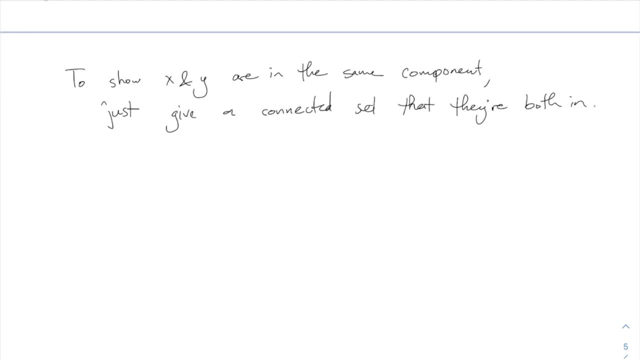 Because that's the definition of component, It's an equivalence class of that weird relation, And the weird relation is defined in terms of There is a connected set Which includes them. So To show that two things are in the same component. 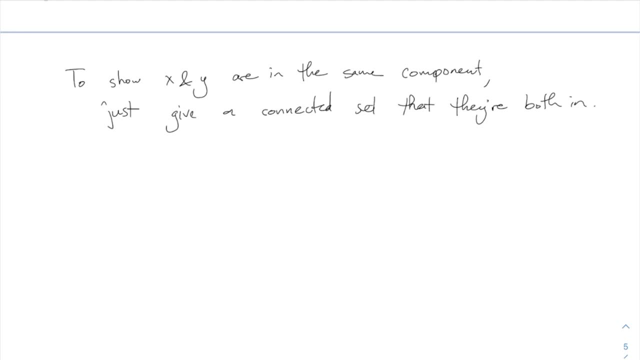 You can just give a connected set That both of those two points are in. To show that they're in a different component Is a little more complicated. You have to show that There can be no connected set Which includes both of those points. 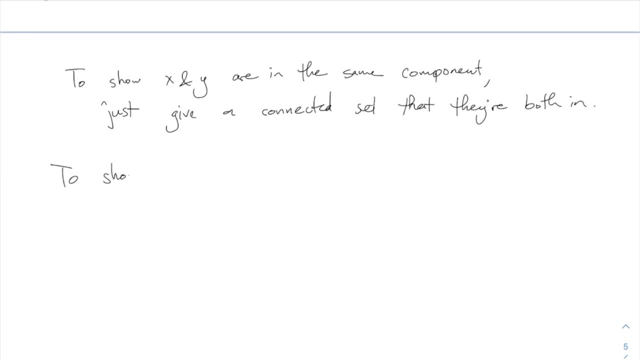 There's sort of a workaround Or a shortcut Or something To show that X and Y Are in different components. We can use A little lemma here, Which I don't want to get into the proof of this. It's obvious enough. 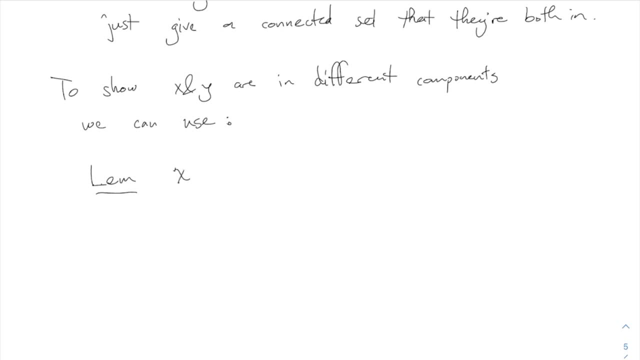 I think that this is true. It says that X and Y Are in different components. This is another way That you can define What the components are. If There exists a separation, X equals U union V. If you can actually. 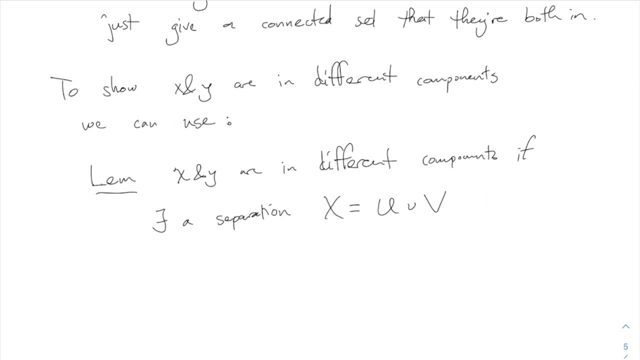 Separate the whole set In such a way That the X is in the U And the Y is in the V. If they end up in different parts of separation, Then they are definitely not In the same component. All right, Like I said, 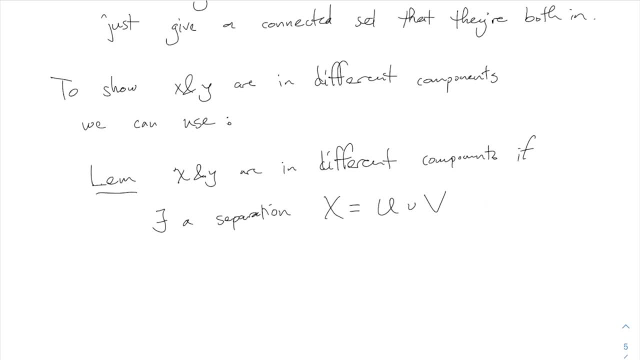 This is actually Another way you could define What the components are, X and Y. If there's a separation like this, where the X and the Y end up sort of on separate sides of the tracks, right, X is in the U and Y is in the B, all right. 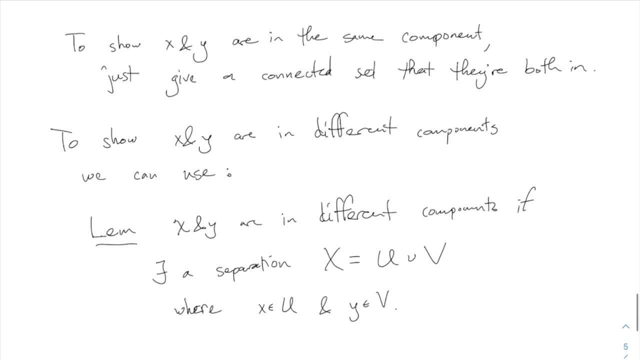 So if you can remember these two basic strategies here- this is how you show the X and Y are in the same component. This is how you show the X and Y are in different components- Then you can pretty much given any example. I would ask you something like: here's an example: 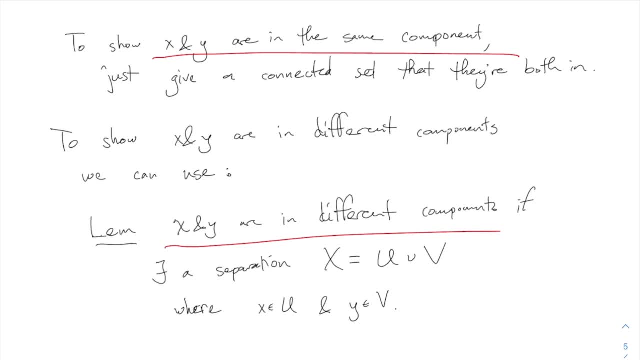 You tell me I could say: are these two points in the same component or not? If you think they're in the same component, you tell me a connected set that they're both in. If you think they're in different components, you give me a separation which puts them in different sides. all right. 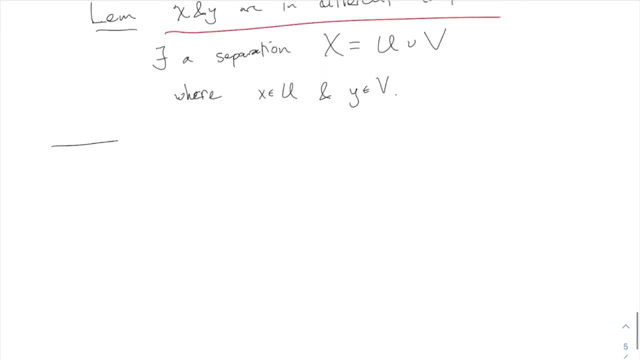 Let's try an example here. How about everybody's favorite disconnected subset of R R minus zero? all right, This is the entire real line, but you take away the point in the middle. This is disconnected into the right side and the left side, all right? 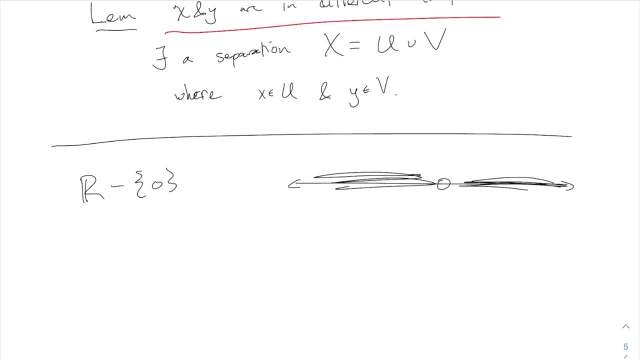 Now, that's obvious enough by looking at the picture, but can we just try and talk about the technicalities a little bit without just sort of saying everything is obvious? I could ask specifically: let's say minus one, one and three, all right. 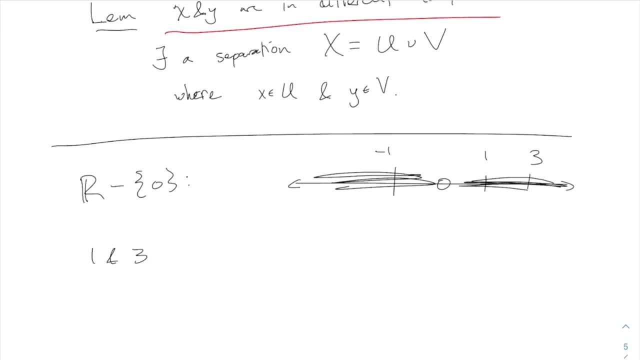 Can you demonstrate that one, One and three are in the same component? I mean, look at the picture, It's obvious. but how do you actually show that? since Remember what I underlined in red above: To show that two points are in the same component, you must. what did I say? 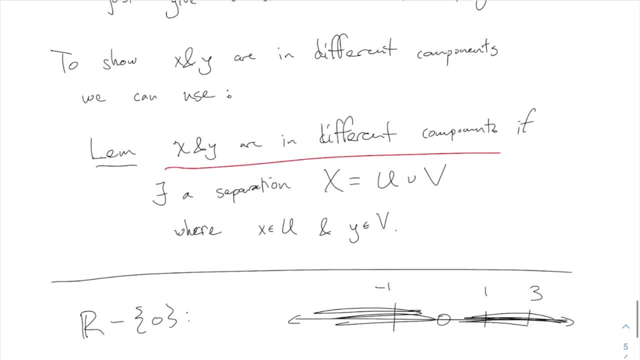 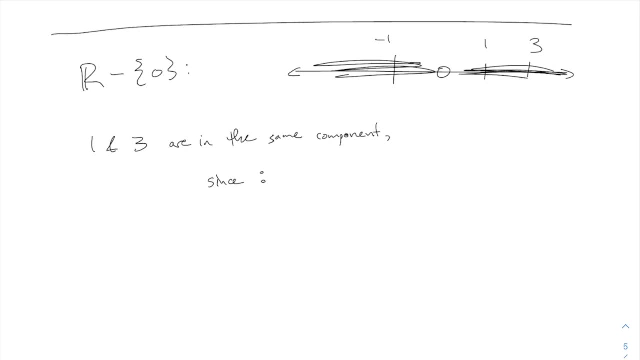 Just give a connected set that they are both in. So can anybody give me a connected set that includes the one and the three? This is not a trick question. Yeah, One half to four, The interval: one half to four, Yeah. 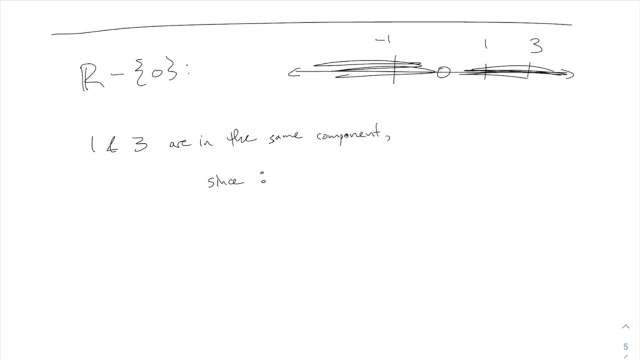 The open interval. Yes, I think she meant the open interval, Although you can use a closed interval too. It just has to be connected, right? It doesn't have to be an open set, just connected. Actually, now that I say it just has to be connected, do you have a better example? 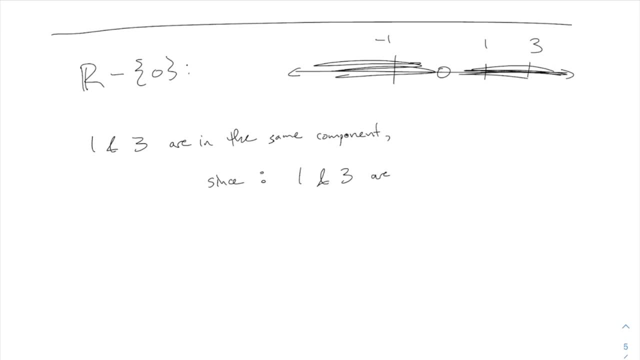 Maybe not. Could it be just the closed interval? Yeah, How about the closed interval one to three? That's the most sort of simple way to do this. One and three are both in. I wrote bath bath in the closed interval one to three. 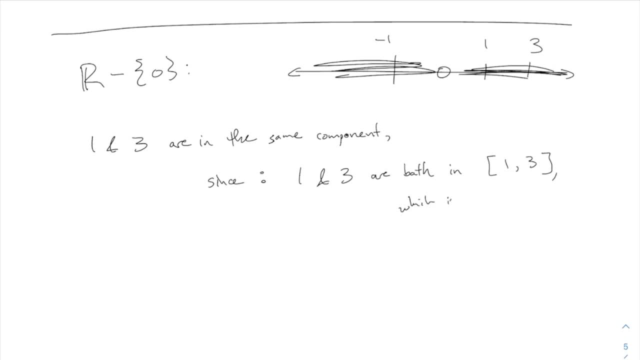 which is connected. All right, So that means one and three are in the same component. What about let's say one and minus one? These are in different components. Now for this. how do you show two points are in different components. 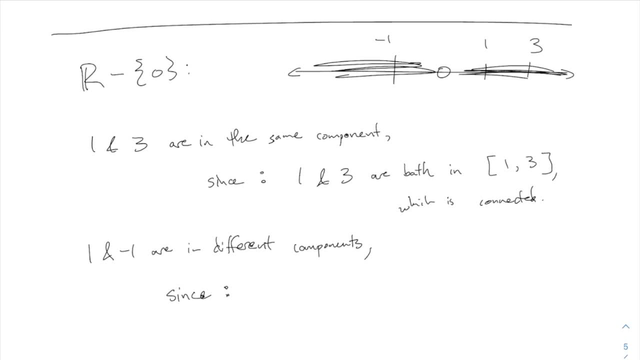 You have to demonstrate a separation of the entire space where one of them ends up in one part and the other ends up in the other part. So if I call this x, since x equals, I'm trying to write a separation here. Can anybody say what separation can I use for x? 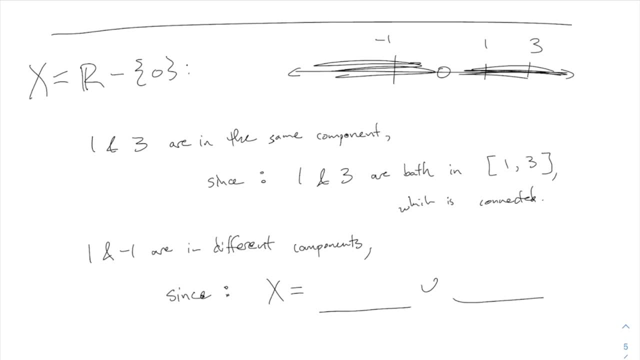 Which, Which makes it so that minus one is on one part and one is on the other part. Actually, there's really only one possibility that you can do here: Yeah, Negative infinity to zero and then zero to infinity. Right Minus infinity to zero and zero to infinity. 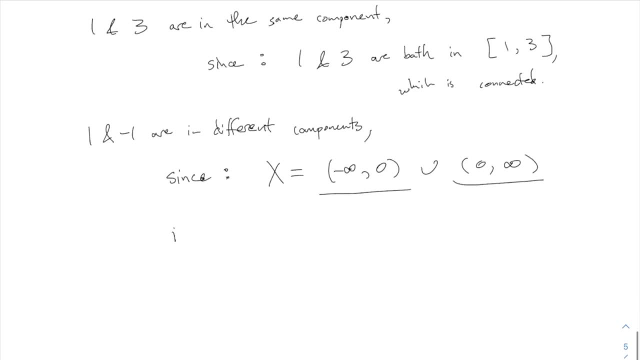 That is a separation. So since x equals, that is a separation of x. Now I suppose technically there's a lot of details you have to check, You have to remember: When you say separation, it means something, something, something. 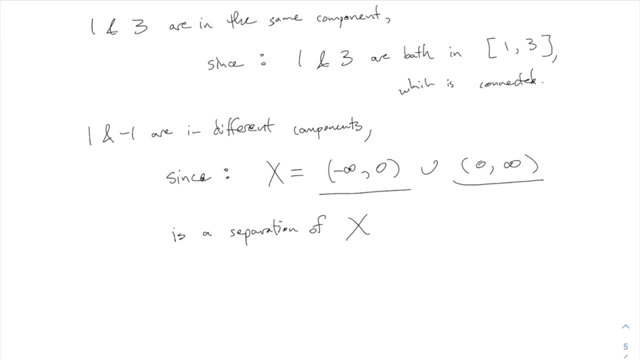 But this is a separation. I hope you, I hope you believe me. So this is a separation and you have to say specifically: one is in the second one, zero to infinity, and minus one is in the other one, right, 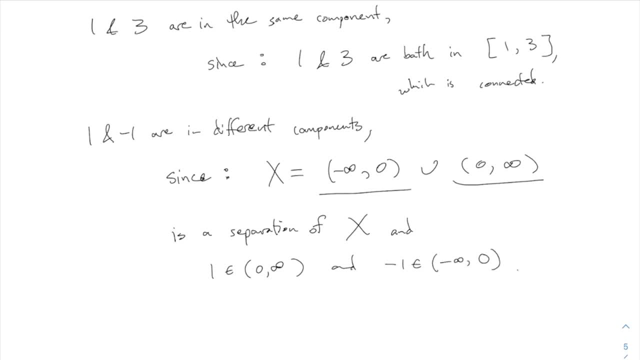 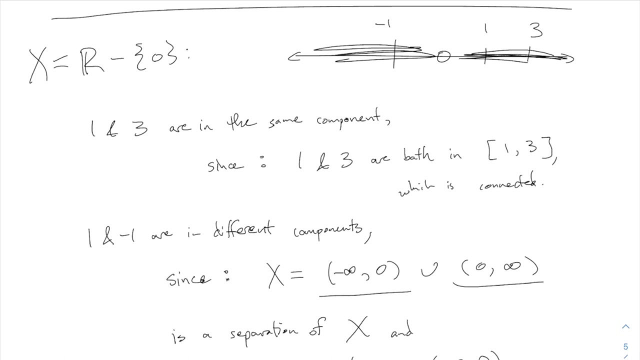 So they are in opposite halves of the separation, and so they are in different components. All right, In fact. so what are the components of this thing? The components are: they are just this part and that part. right, Two points that are in one side will be in the same component. 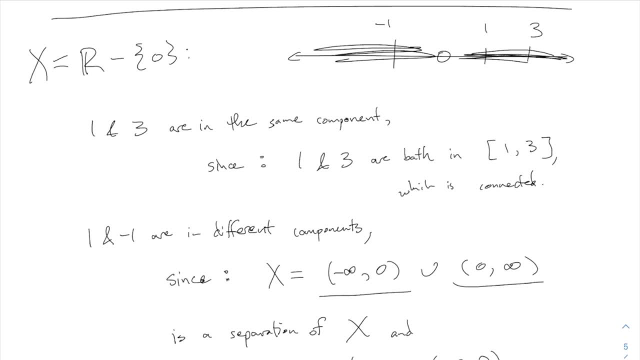 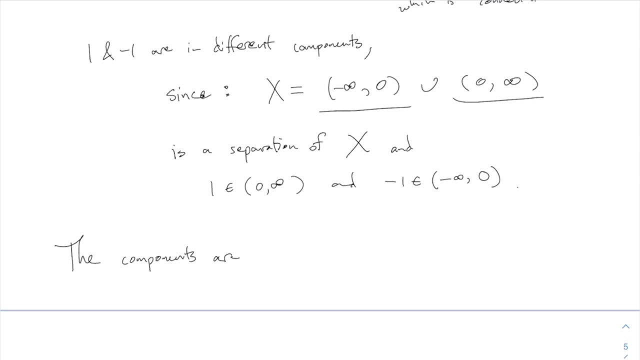 Two points on the other side will be in the same component, and if you have one from one and the other, they're in different components. So in this example the components are. they are just minus infinity to zero and zero to infinity. 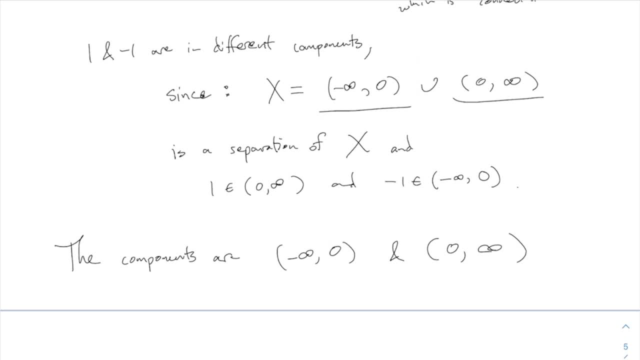 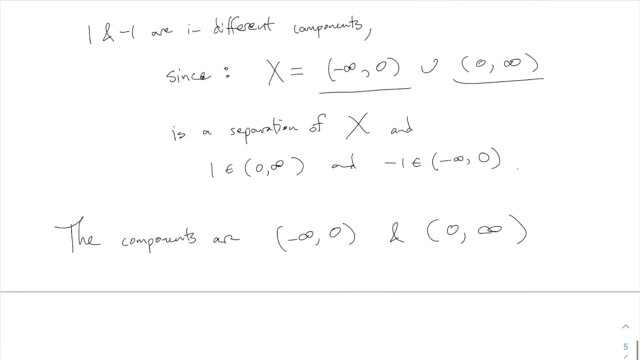 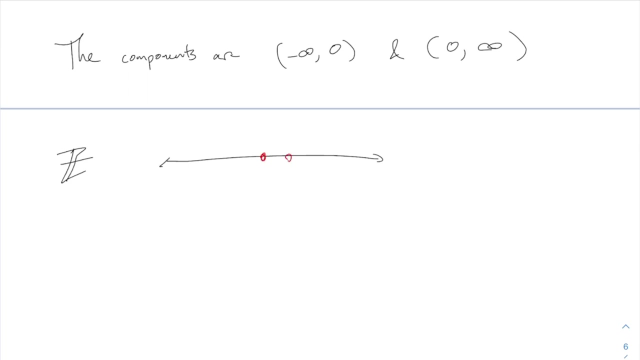 All right, There are two components and that's what they are. All right, What about we have five more minutes? I got two more examples, maybe one and a half. How about another subset of R Z? So this is only the integer points inside the real line. 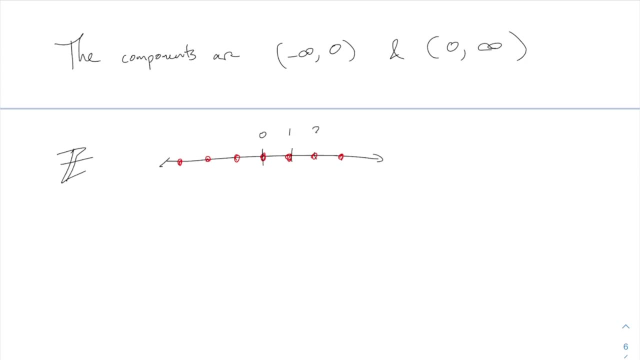 All right, Maybe I have zero, one, two et cetera. What are the components? You could ask yourself a preliminary question. For example, very specifically, are one and two in the same component? Anybody have a thought about that? 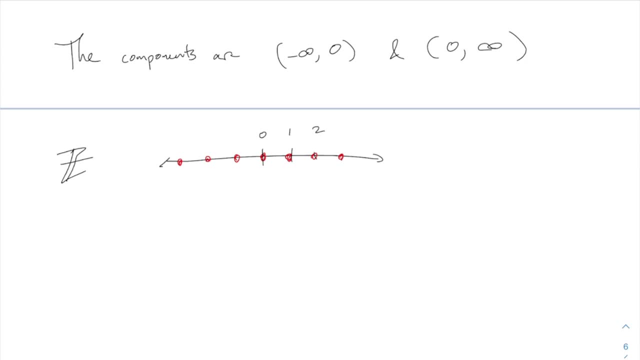 I think the answer is no. One and two are not in the same component. because, well, why not? You should write a separation, if you really believe that, which I do. One and two are not in the same component. The same component, the same component, since I can make a separation something, union something. 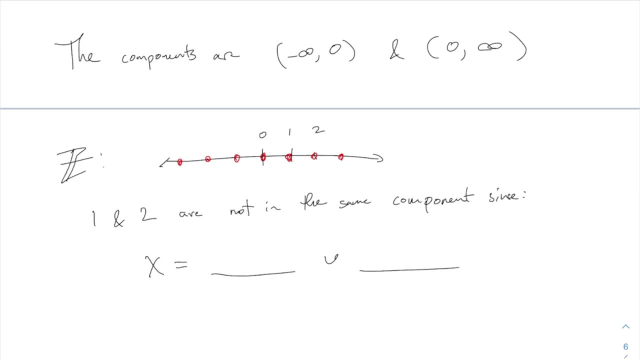 Anyone. can anyone tell me a separation here? It has to be two open sets that satisfy blah blah, blah, blah blah. This is slightly weird. When I say open sets, you might get a little nervous. You got thoughts. 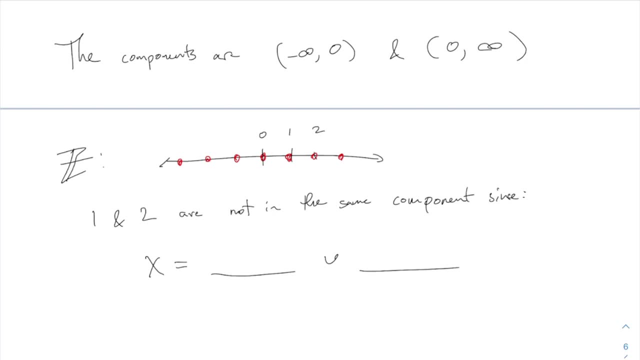 Can you do negative infinity to one- because that's Uh-huh, I like this- Minus infinity to one, Would you? I'm going to go to two. This is not quite right, but I'm going to. So one thing I like. I like that you said something. intersects z. 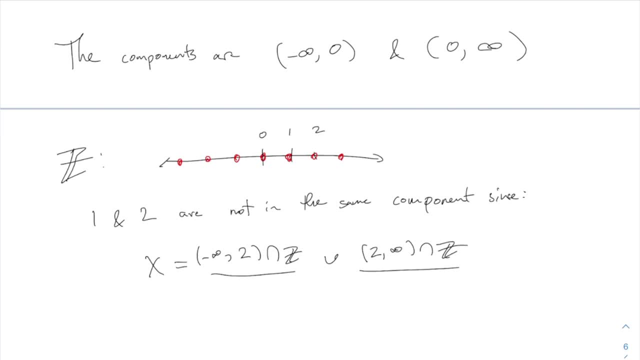 You're trying to make open sets in here with the subspace topology, And that's what open sets in the subspace topology should look like. It should look like an open interval from r intersected with z. So these two things, they really are two open sets which are supposed to cover the whole thing. 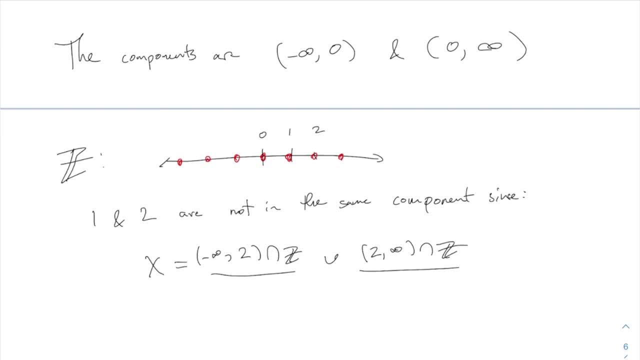 And one is in one of them and two is in the other. one, right? That actually is technically not true of this. One is in this one, but two is not in this one. Can you modify your? I want to make it so that one is in here and two is in here. 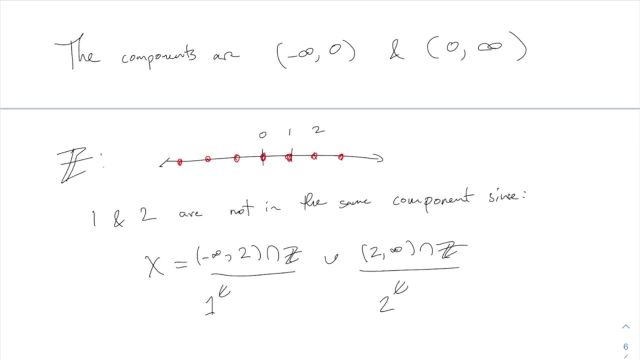 Although right now. No, that's not true. Two is not in that one because of this open side. Anyone have an idea to remedy the situation? Yeah, Change the two to a one. Yeah, that would work This over here. just make it a one. 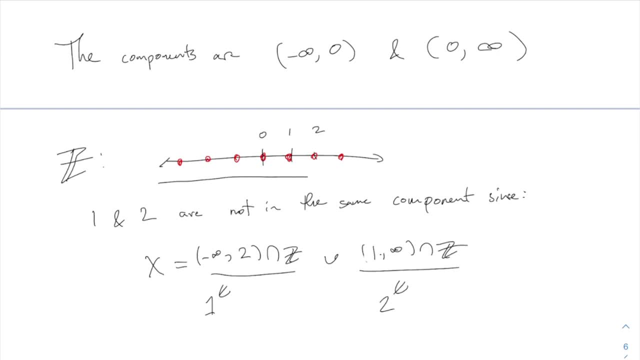 So if you were to draw these intervals, it would look like this, and then this: Now it looks like they overlap, which you don't want, But once you intersect them with z, they don't overlap anymore. And so everything. Everything is fine now, right. 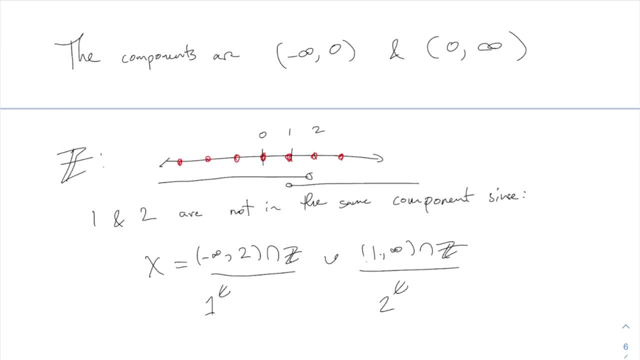 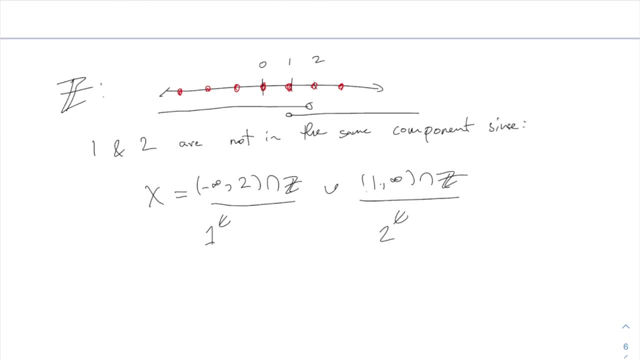 They do overlap as real intervals, but I'm intersecting them with z, So really they don't have any intersection in the subspace. all right, Yeah, great, So one and two are not in the same component. What can anybody say? 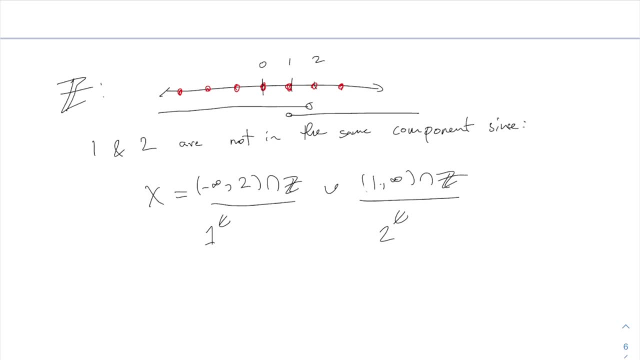 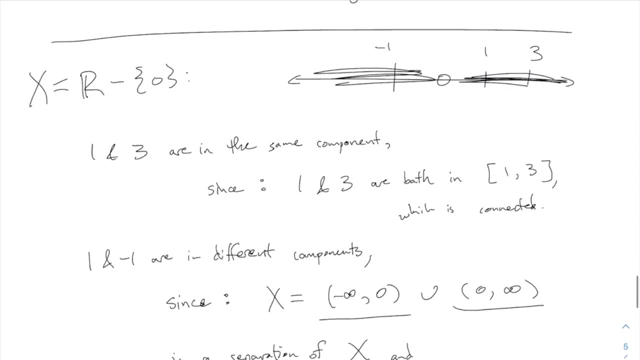 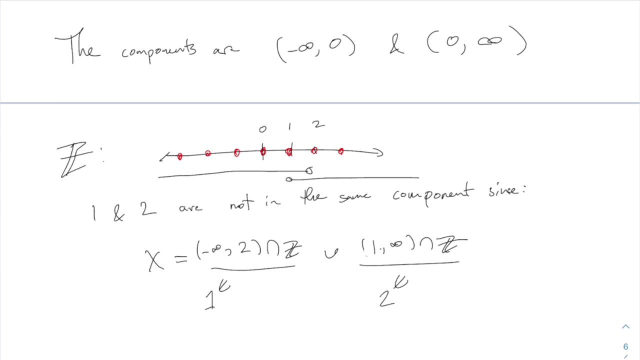 What are the components here? You should be able to say: the components are what You could describe them in words, or something Like in our previous example. the components were these, These two pieces. There were two components in this one. Can anyone say like how many components are there? 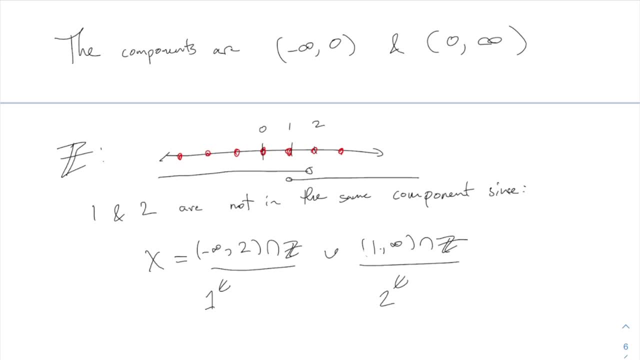 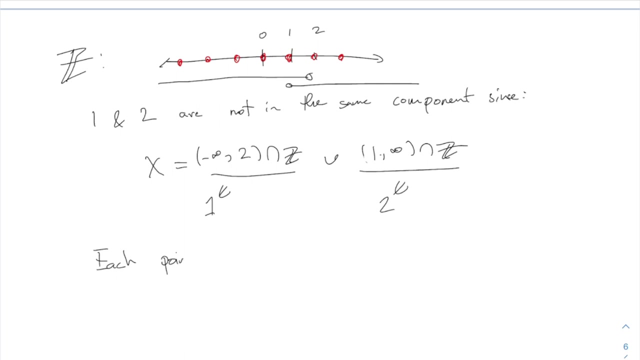 And what are they? Yeah, Is like every integer a component. Yeah, each number by itself is a component, right, And there are infinitely many components in this case. So here I would say: each point by itself is a component. 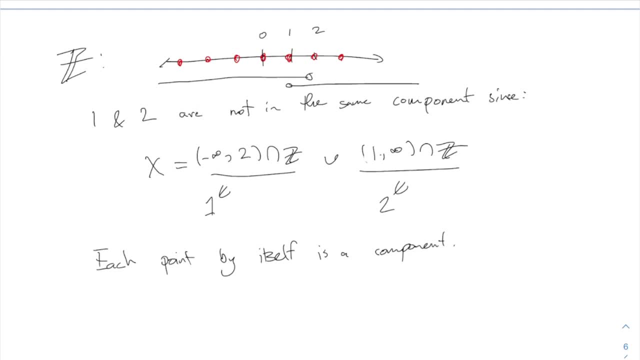 All right, So z has infinitely many components. Yeah, great, Actually, there's a word for this. When each point by itself is a component, this is kind of in terms of connectedness, this is sort of like the worst case scenario.